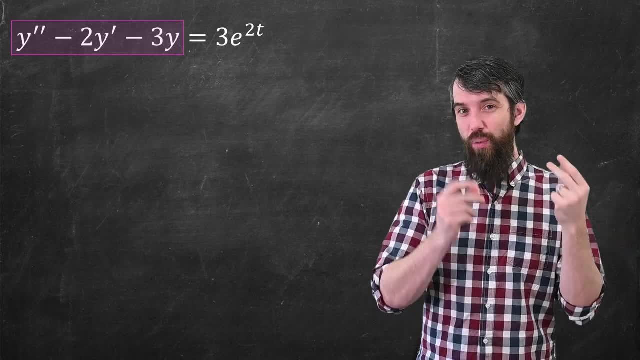 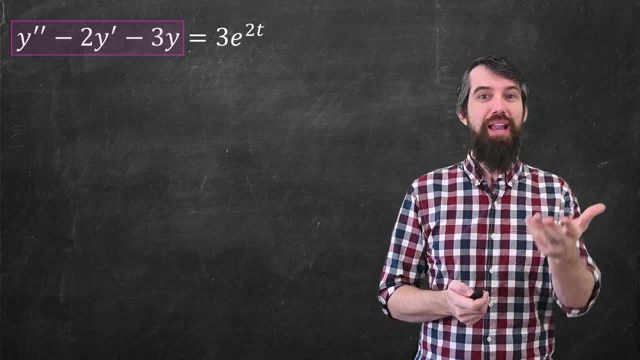 the various terms y, y prime and y double prime. But when we study constant coefficients, thus far the right hand side has always been zero, what we call homogeneous. But now I want to figure out how do I deal if the right hand side is not zero, if it's some other function of the independent 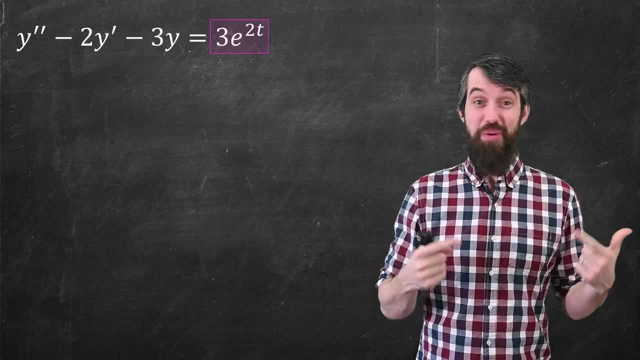 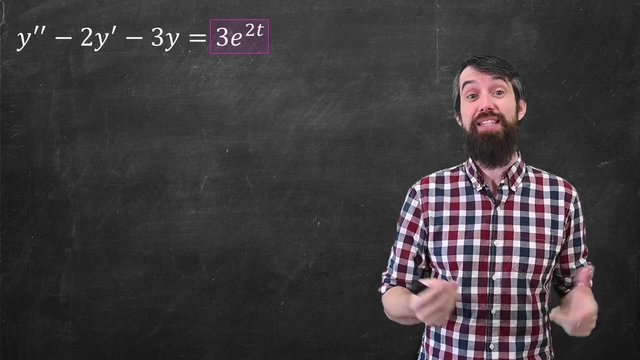 variable like 3e to the 2t. What do I do there? So, as you can probably tell, this video is part of an entire series on differential equations. The link to the playlist and the free and open source textbook that accompanies it is down in the description, So I'd encourage you to check. 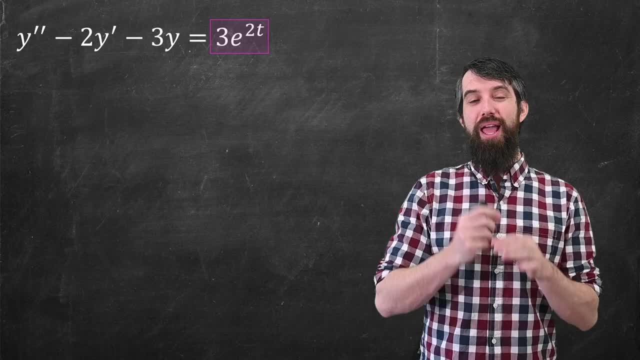 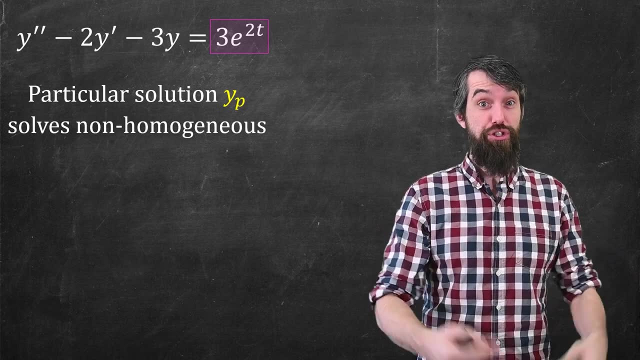 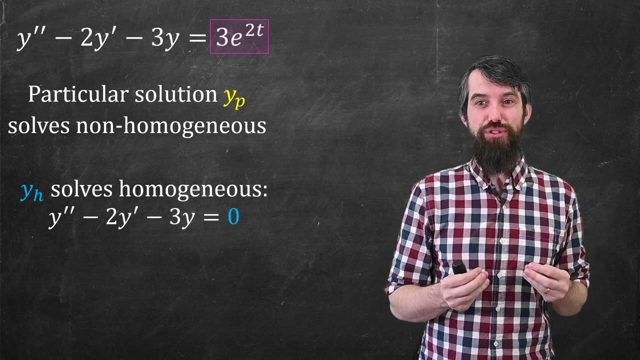 that out. Okay, so some terminology. first I'm going to call a particular solution, y sub p, for particular to be just any solution, not the general solution, not all possible solutions, just any one that you so wish. And then I'm going to let y sub h be the general solution to the same. 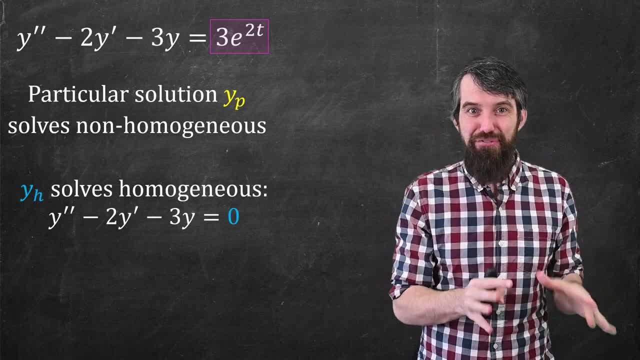 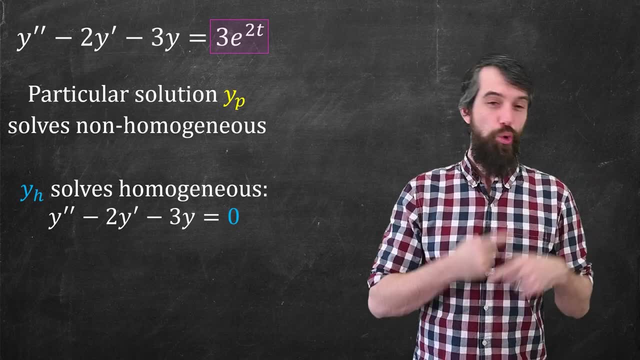 equation if it was homogeneous. So you keep the left hand side, but you just set the right hand side being equal to zero, which is indeed a type of equation that we know how to solve. So y of h is the general solution, which means it has constants, and y of p is just any one particular. 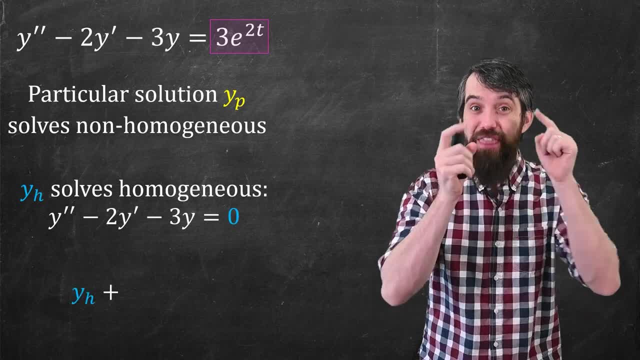 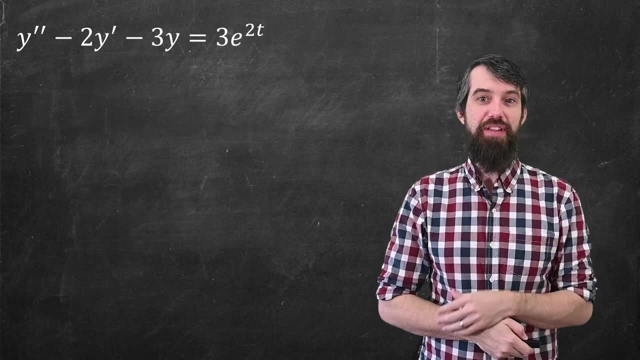 solution. Now, if you're going to be able to solve this problem, you're going to have to do a lot of thinking. So I want to consider what happens if I add those two things together: the homogeneous solution plus the particular. Well, I can just plug this in, So let me take the left hand side. 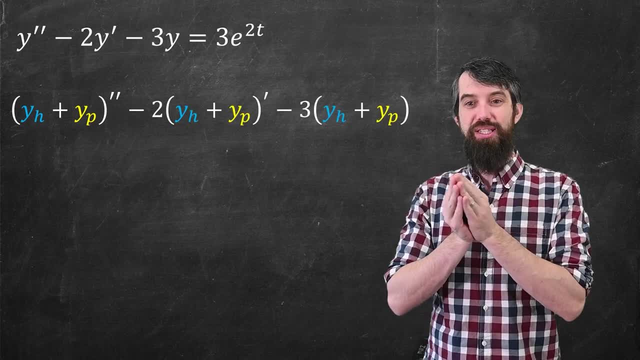 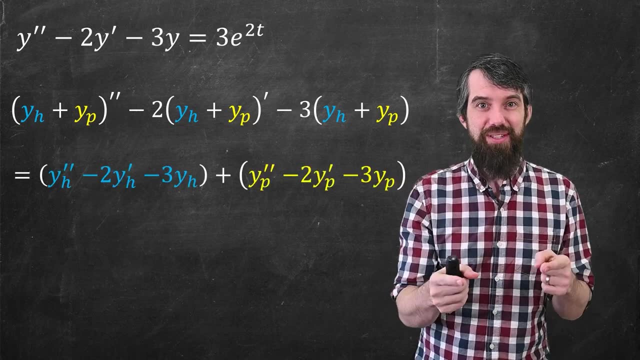 and everywhere. I'm going to plug in the homogeneous plus the particular solution. So two derivatives of that thing minus two times, one derivative of that minus three times, just plug it in. And then what? I notice that I can separate the two different sides. I can put everything with. 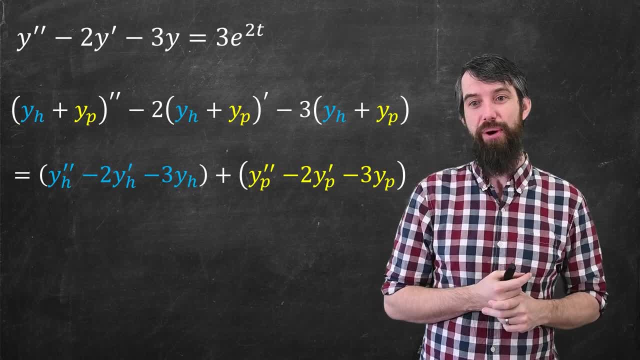 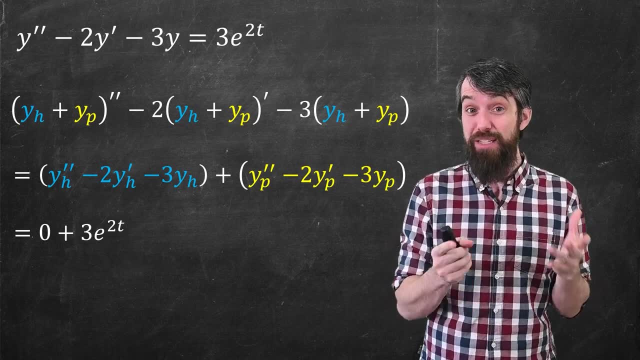 the homogeneous solution together and everything with the particular solution together. But this just looks like the left hand side of the differential equation For the homogeneous- since this is a solution to the homogeneous, we know that portion adds up to zero. And then for the particular, the particular solves the non-homogeneous, So that portion adds. 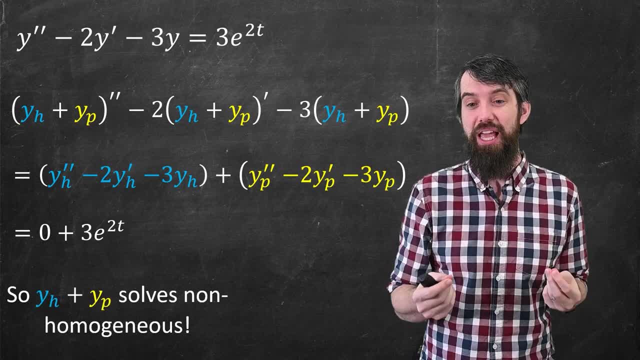 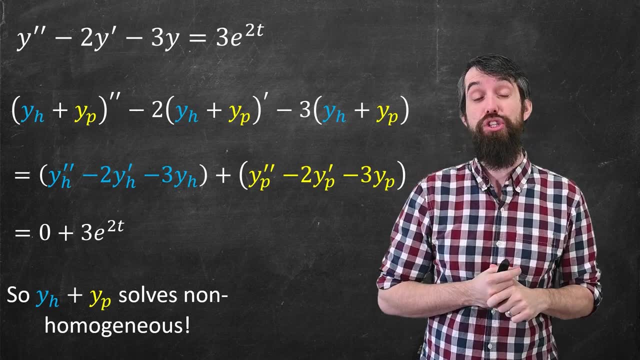 up to 3e to the 2t, which of course is just 3e to the 2t, And thus the homogeneous plus the particular. that is a solution to the non-homogeneous equation. So here's the idea. If you 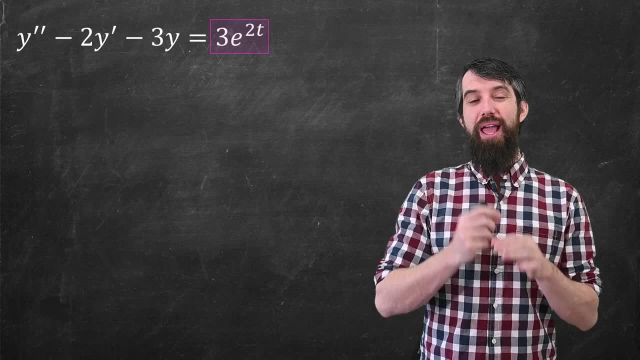 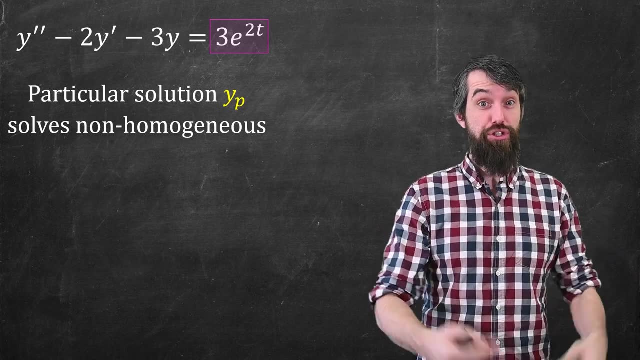 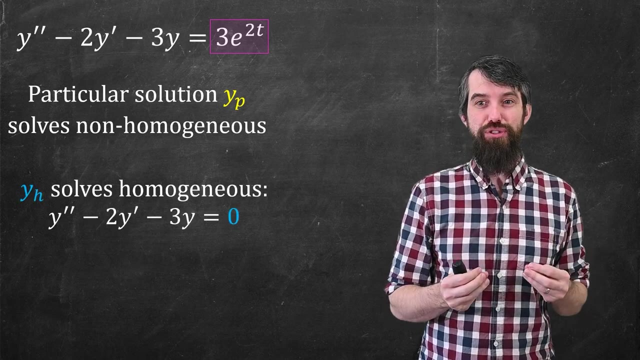 that out. Okay, so some terminology. first I'm going to call a particular solution, y sub p, for particular to be just any solution, not the general solution, not all possible solutions, just any one that you so wish. And then I'm going to let y sub h be the general solution to the same equation, if 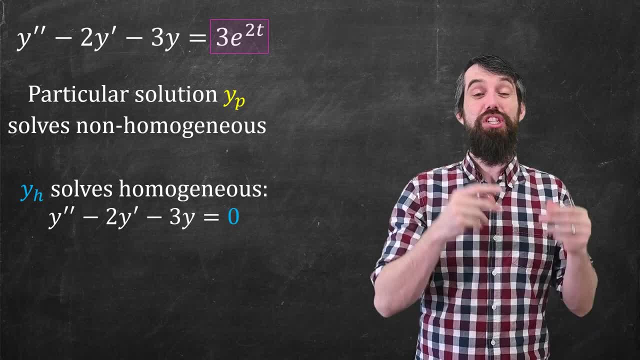 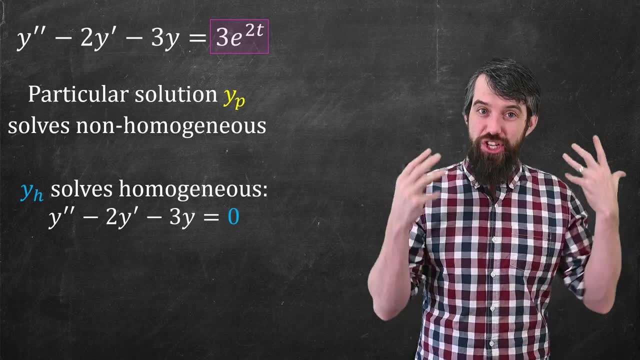 it was homogeneous. So you keep the left hand side, but you just set the right hand side being equal to zero, which is indeed a type of equation that we know how to solve. So y of h is the general solution, which means it has constants, and y of p is just any one particular solution. Now, 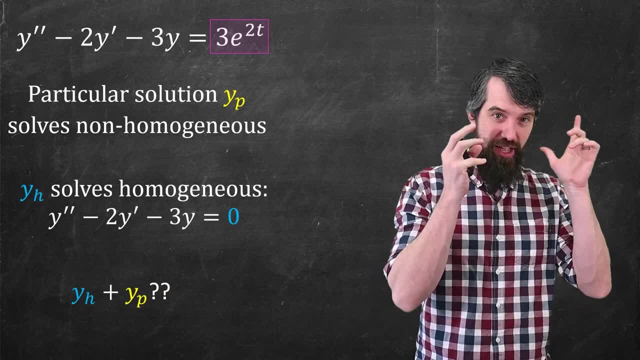 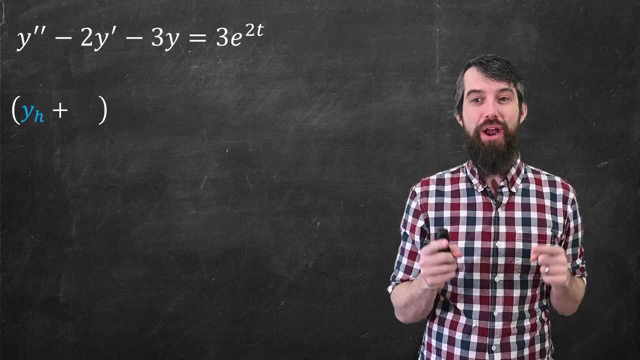 I want to consider what happens if I add those two things together: the homogeneous solution plus the particular. Well, I can just plug this in. So let me take the left hand side and everywhere I'm going to plug in the homogeneous plus the particular solution. So two derivatives of that. 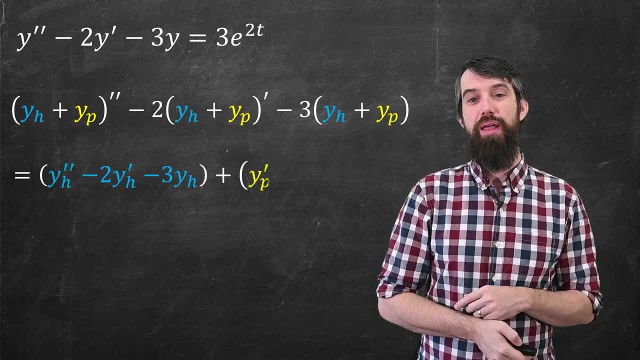 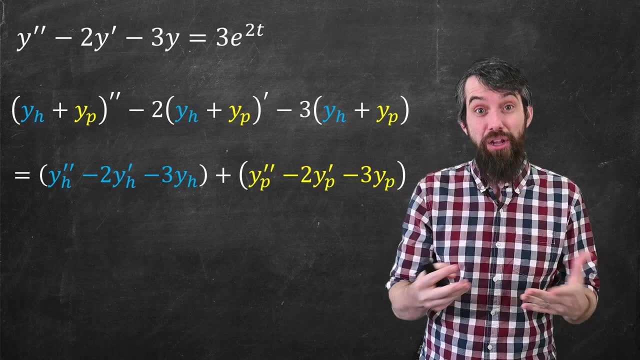 thing minus two times, one derivative of that minus three times. just plug it in And then what I note is that I can separate the two different sides. I can put everything with the homogeneous solution together and everything with the particular solution together, But this just looks like the 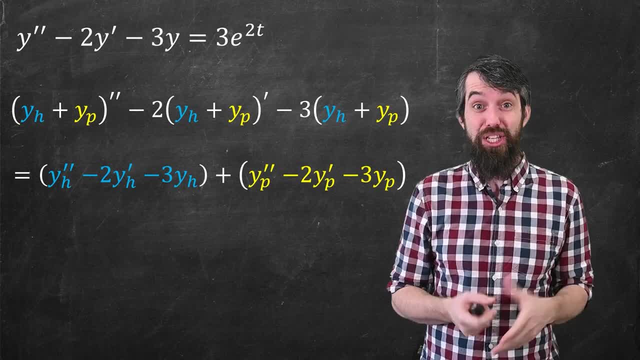 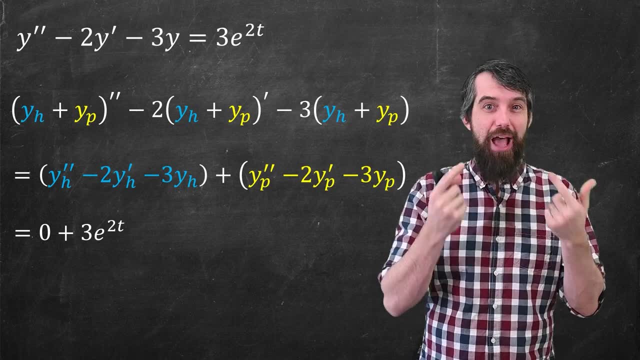 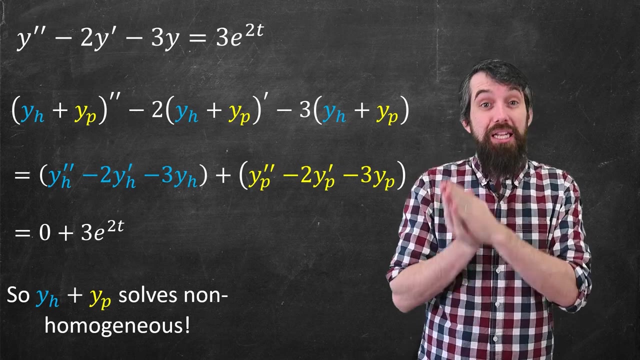 left hand side of the differential equation For the homogeneous. since it's a solution to the homogeneous, we know that that portion adds up to zero. And then, for the particular, the particular solves the non-homogeneous, so that portion adds up to 3e to the 2t, which of course is just 3e to the 2t, And thus the homogeneous plus the. 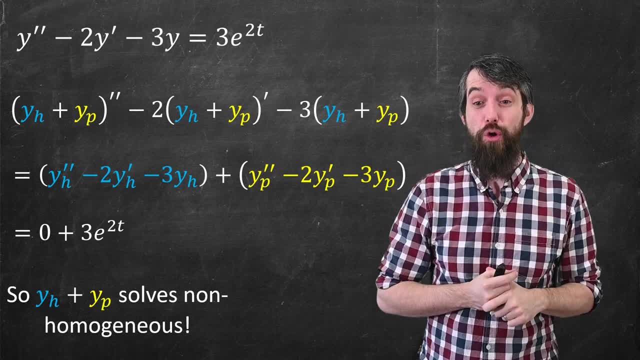 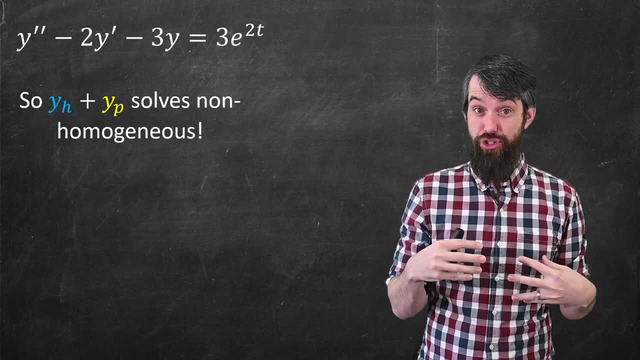 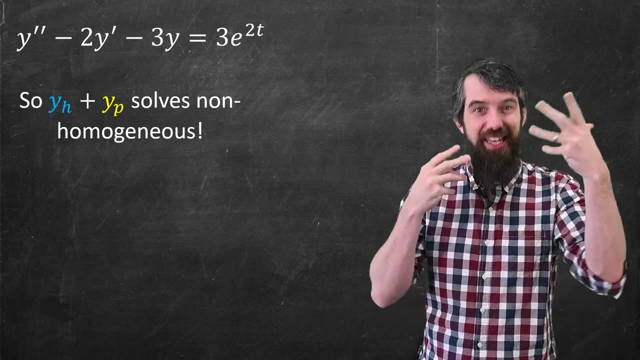 particular. that is a solution to the non-homogeneous equation. So here's the idea: If you have a particular solution and I have a homogeneous solution, we can add our solutions together and that still solves the non-homogeneous equation. That's another solution to the non-homogeneous 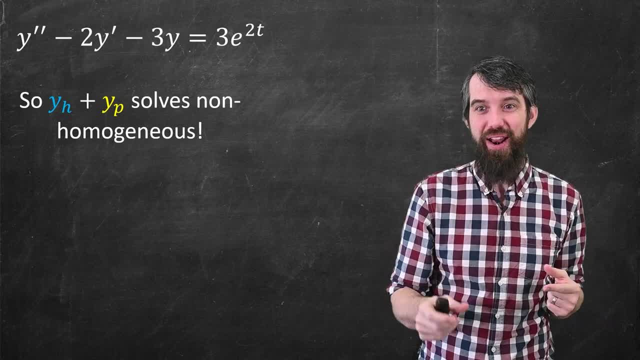 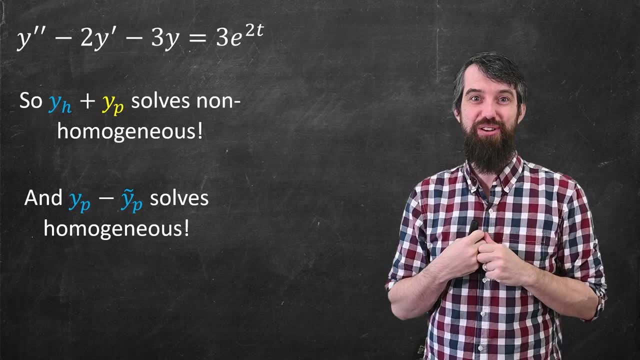 equation. I can actually do the same thing with a slight twist on it. Let me imagine that there are two different, particular solutions. I have a particular solution, yp, and you have a particular solution. perhaps we'll call it y tilde sub p. Well then, how much can you- and I disagree, I mean we. 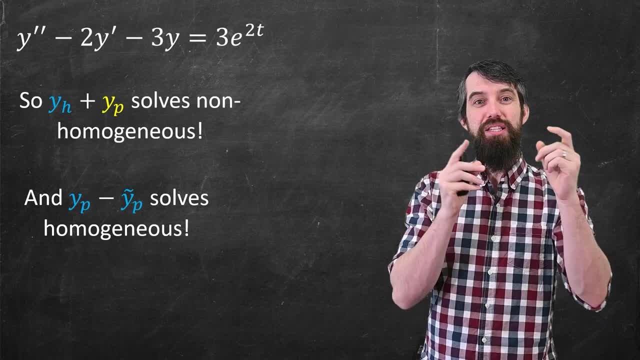 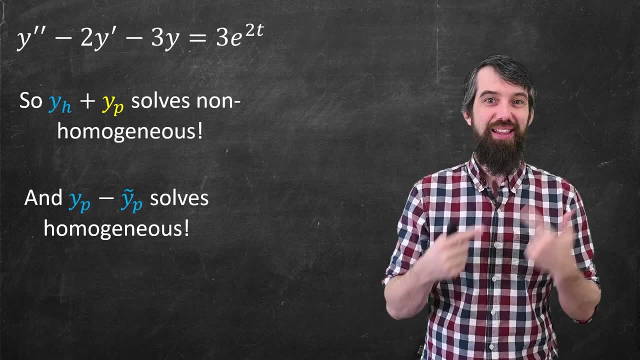 can disagree a little bit, but the difference between you and I is a solution to the homogeneous. Again, I can prove this by plugging it in and seeing that it would add up to zero. Indeed, you can plug this into the left hand side and you'd get that adding up to 3e to the 2t, minus 3e to the 2t, which would 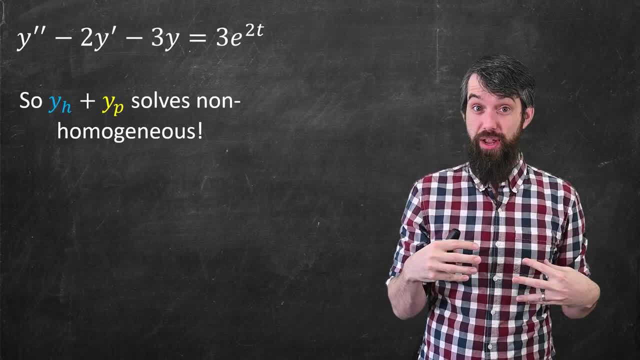 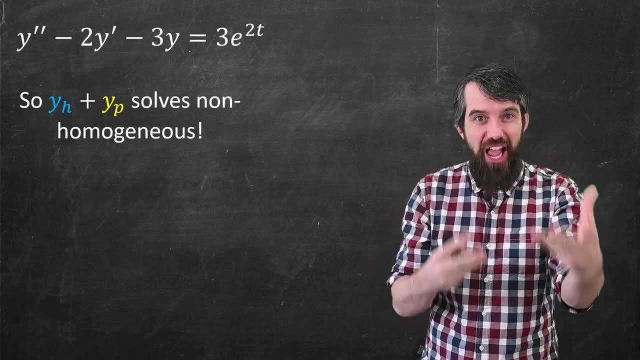 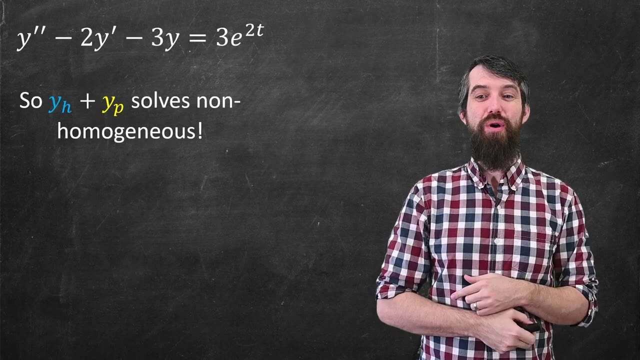 have a particular solution and I have a homogeneous solution. we can add our solutions together and that still solves the non-homogeneous equation. That's another solution to the non-homogeneous equation. I can actually do the same thing with a slight twist on it. Let me imagine that there are 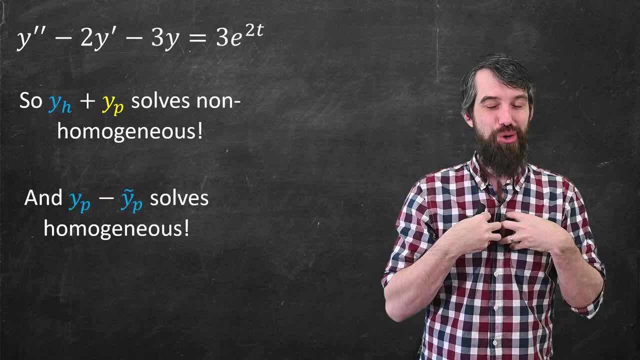 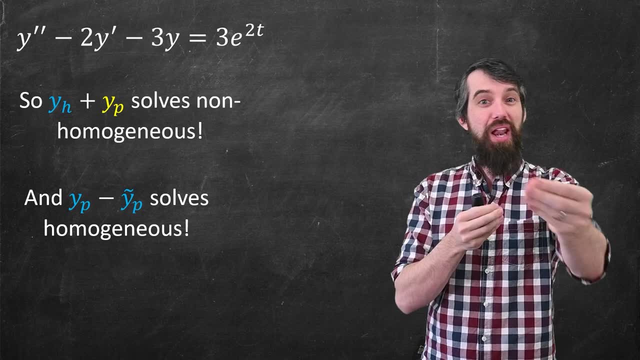 two different particular solutions. I have a particular solution, yp, and you have a particular solution. perhaps we'll call it y tilde sub p. Well then, how much can you and I disagree? I mean, we can disagree a little bit, but the difference between you and I is a solution to the homogeneous. 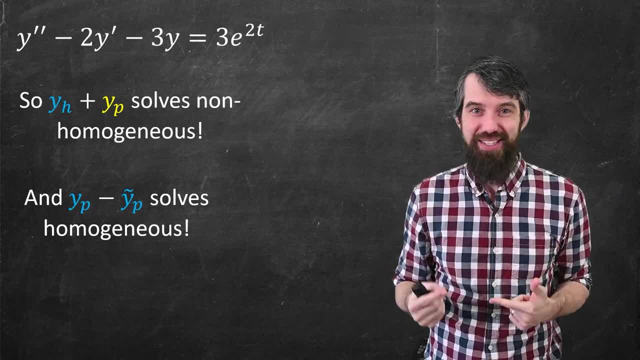 And we can prove this by plugging it in and seeing that it would add up to zero. Indeed, you can plug this into the left-hand side and you'd get that adding up to 3e to the 2t minus 3e to the 2t, which. 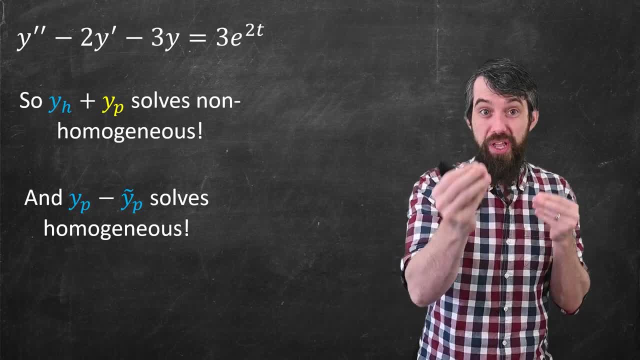 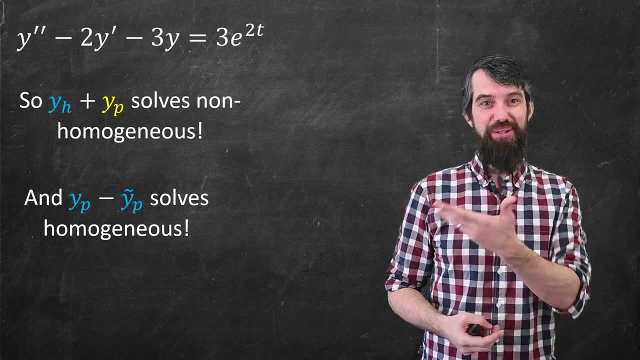 would just be zero. It's a solution to the homogeneous. So you and I can disagree only by a solution to the homogeneous. So this is going to give us a methodology. Basically, we're going to find the general solution to the homogeneous. We're going to find any particular solution. you. 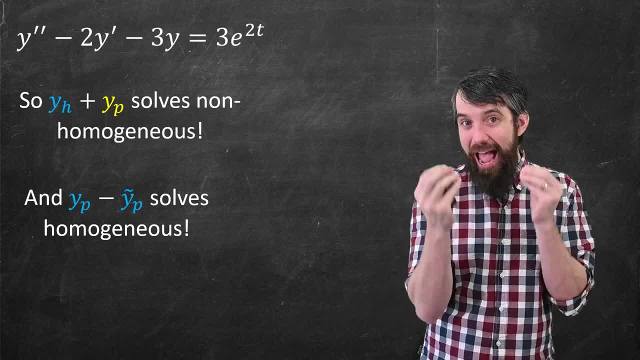 wish. It doesn't have to be anything fancy, just whatever one you like, And then, if you add those together, you get all the solutions, solutions. So let me show you how this is going to work. So, step one: I'm going to solve the. 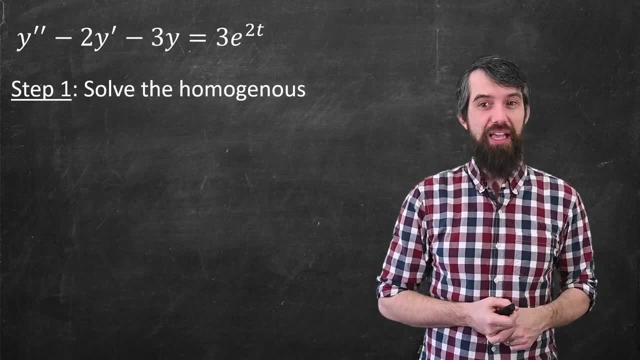 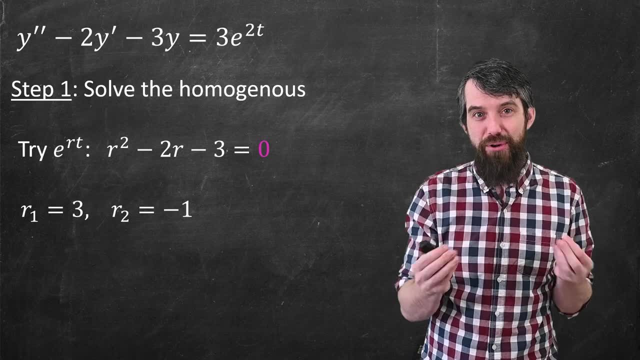 homogeneous. This is something that we know how to do from our past, so we'll do it quickly. You plug in e to the rt, you get the characteristic equation, you solve for the roots of that characteristic equation and you write the general solution to the homogeneous system as c1. e to the 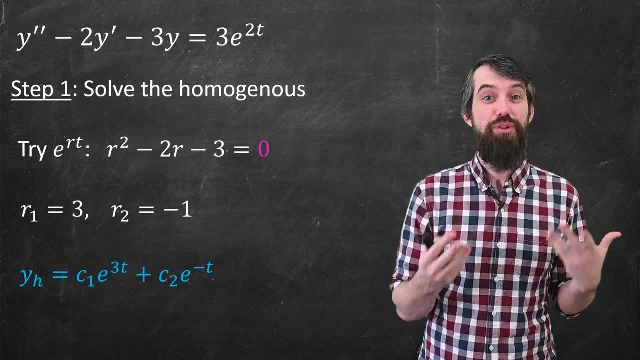 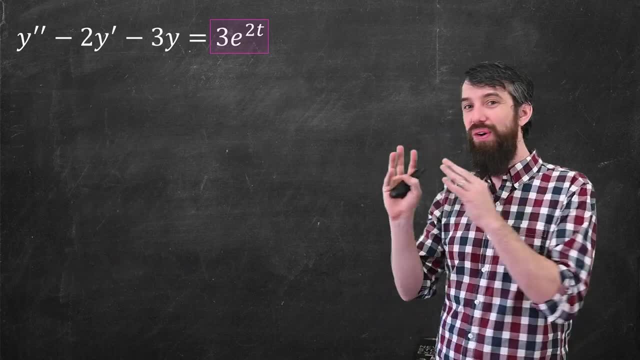 3t and c2 e to the minus t, because you have these two roots, 3 and minus 1.. Okay, that's the old part, but now we move on to step two, where we look particularly at the non-homogeneity. the 3e. 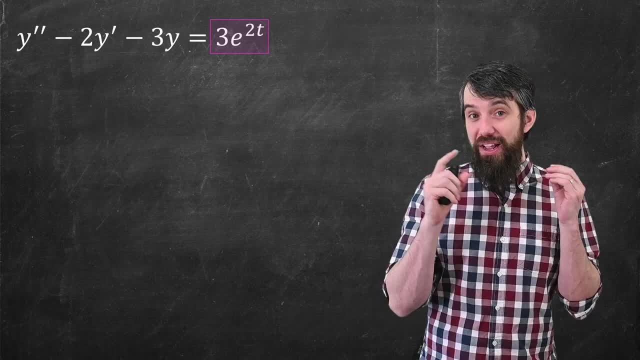 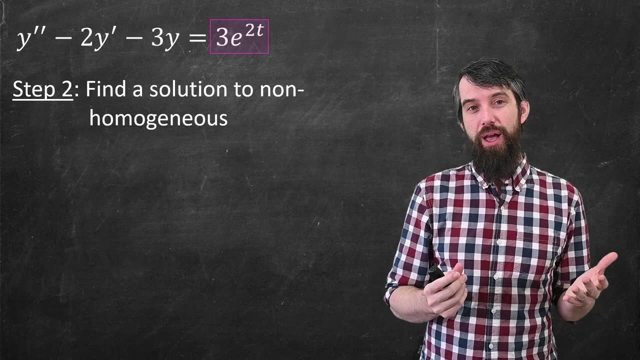 to the 2t part. So what I want to do is I want to find a solution- any solution, one solution doesn't have to be all of them- to the non-homogeneous equation. What I'm going to do is: 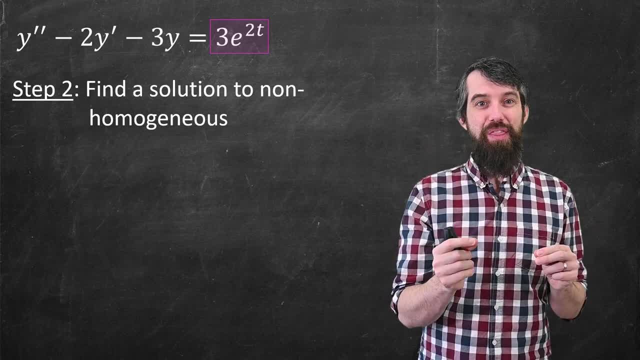 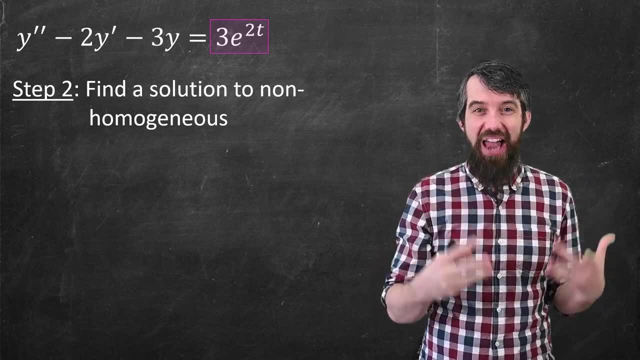 I'm going to do a guess. I'm going to guess that the answer looks kind of like the right-hand side, kind of like 3e to the 2t, but because this is called the method of undetermined co-efficient, you might guess that my coefficient will be undetermined. So what I mean by this is: 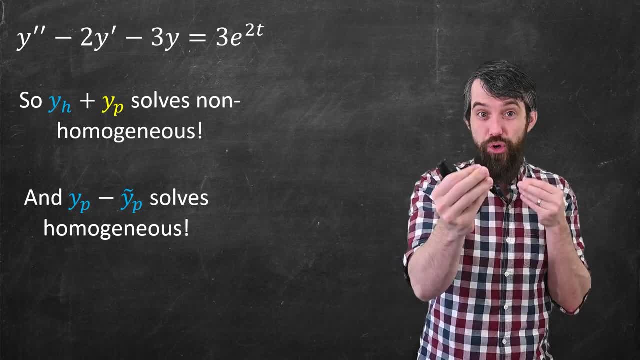 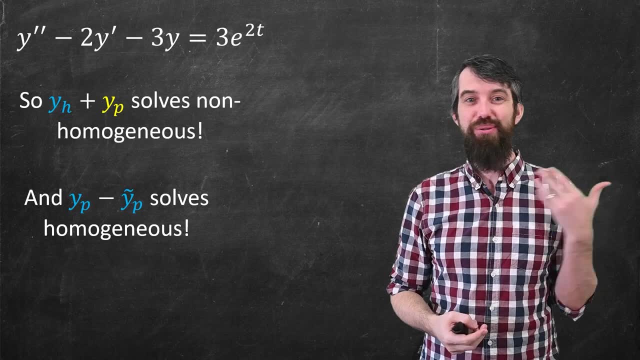 just be zero. It's a solution to the homogeneous. So you and I can disagree only by a solution to the homogeneous. So this is going to give us a methodology. Basically, we're going to find the general solution to the homogeneous. We're going to find any particular solution you wish, Doesn't? 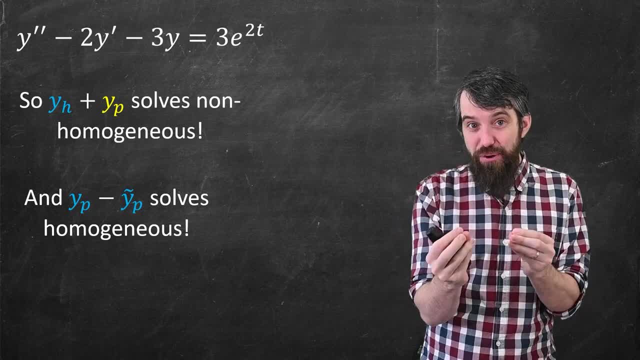 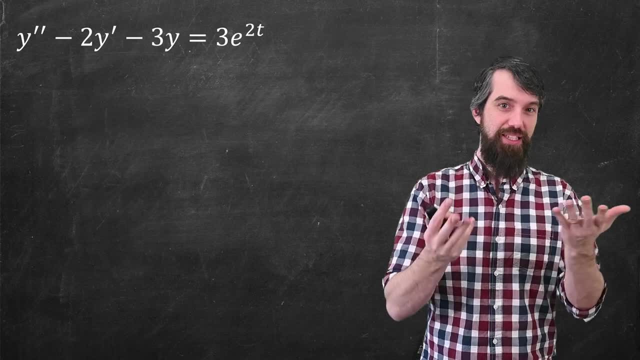 have to be anything fancy, just whatever one you like, And then, if you add those together, you get the solutions. So let me show you how this is going to work. So, step one, I'm going to solve the homogeneous. This is something that we know how to do from our past, so we'll do it quickly. 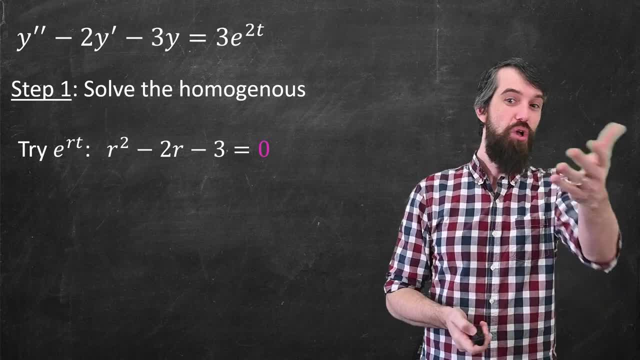 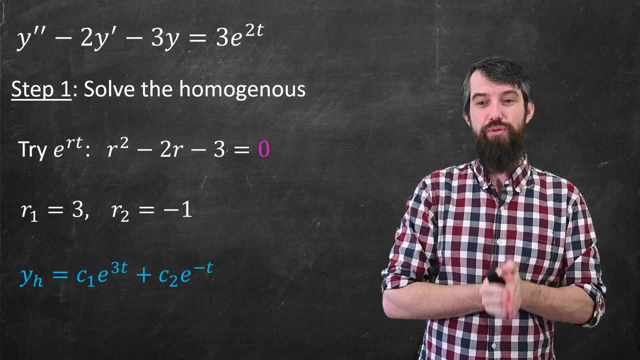 You plug in e to the rt, You get the characteristic equation, You solve for the roots of that characteristic equation and you write the general solution to the homogeneous system as c1 e to the 3t and c2 e to the minus t, because you have these two roots, 3 and minus 1.. Okay, that's the old part. 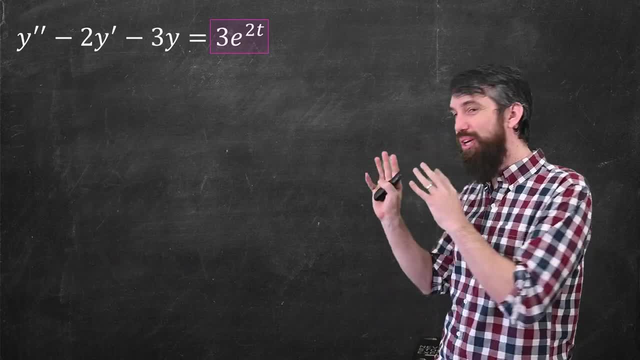 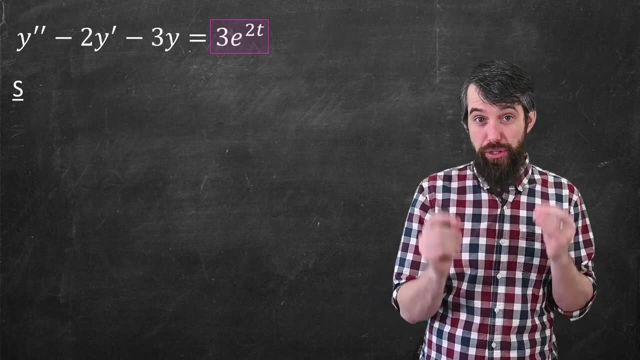 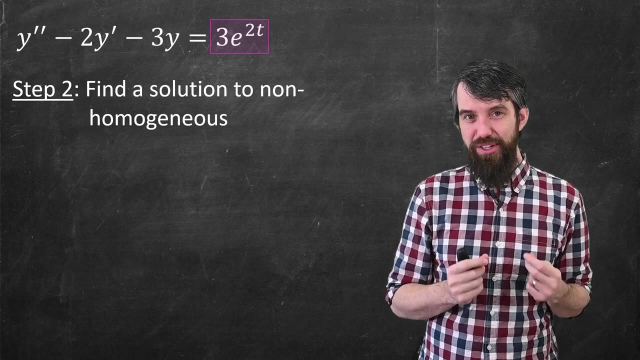 But now we move on to step two, where we look particularly at non-homogeneity, The 3e to the 2t part. So what I want to do is I want to find a solution- Any solution, One solution Doesn't have to be all of them- To the non-homogeneous equation. And what? 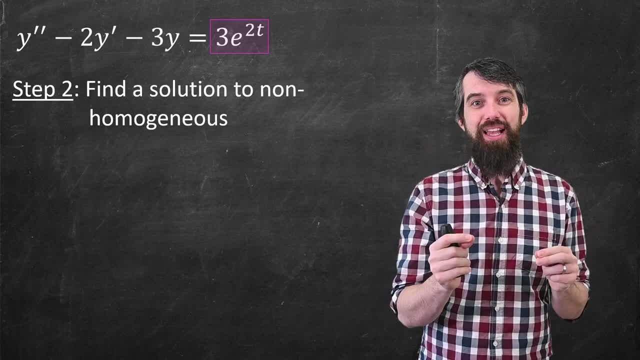 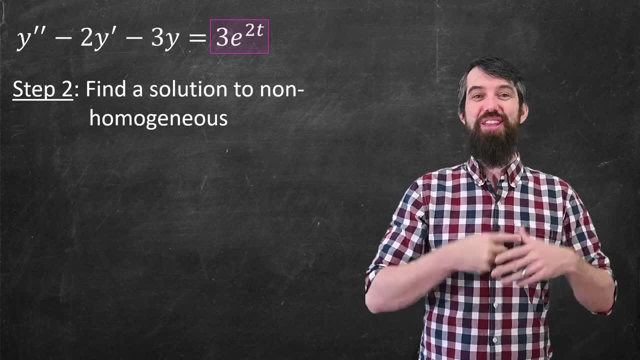 I'm going to do is. I'm going to do a guess. I'm going to guess that the answer looks kind of like the right hand side, Kind of like 3e to the 2t, But because this is called the method of, 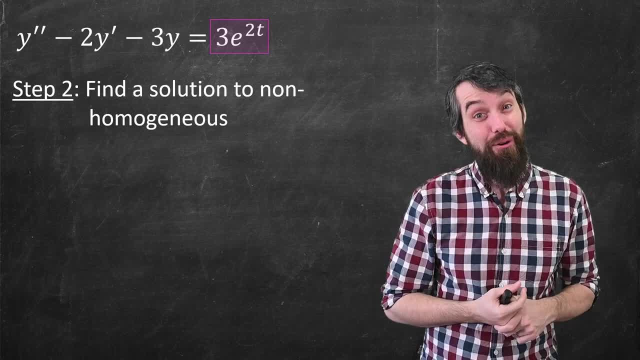 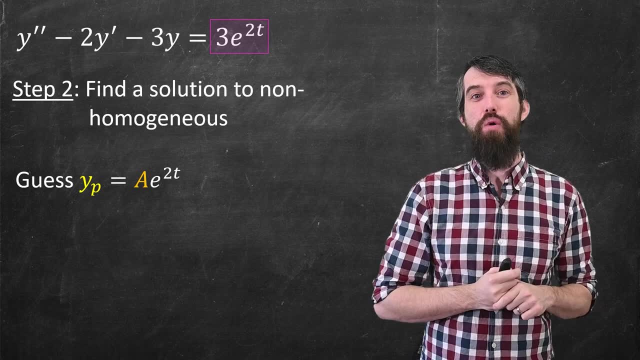 undetermined coefficients. you might guess that my coefficient will be undetermined, So my guess is. here's my guess: Instead of the three, I put an undetermined coefficient, a. But other than that, I leave the same structure. The e to the 2t is going to be the same. So my guess is: 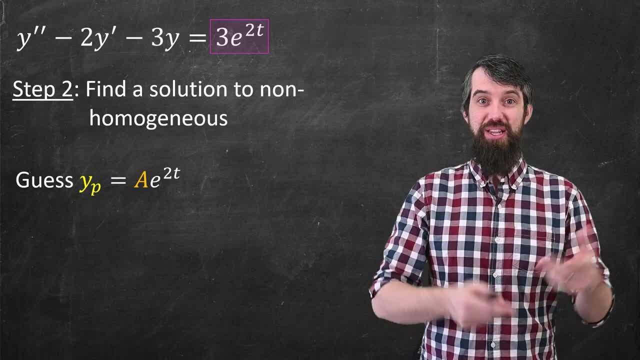 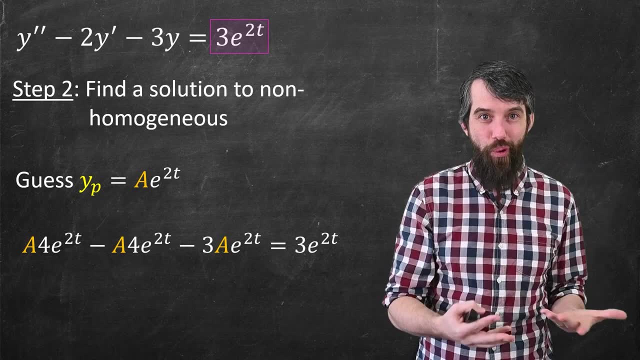 that some constant a times e to the 2t. I mean, it's a guess, So let's just plug it in. Well, if I do that, then Okay, two derivatives of this is going to give 2 times 2 is 4 times 1 to the 2t. 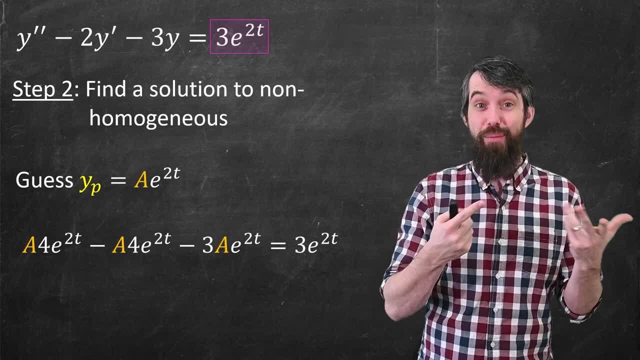 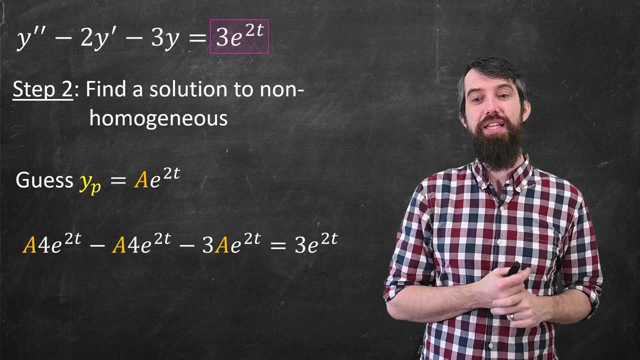 Then minus 2 times 2 e to the 2t, So now minus 4 times a e to the 2t. And then finally minus 2 times a e to the 2t, 3y minus 3a e to the 2t, So just a lot of e to the 2t's everywhere. Then observe, well, I have a plus. 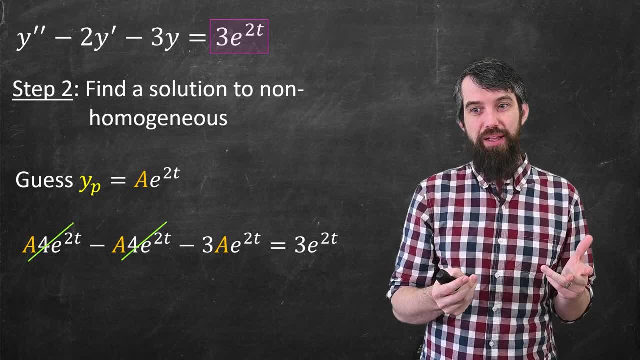 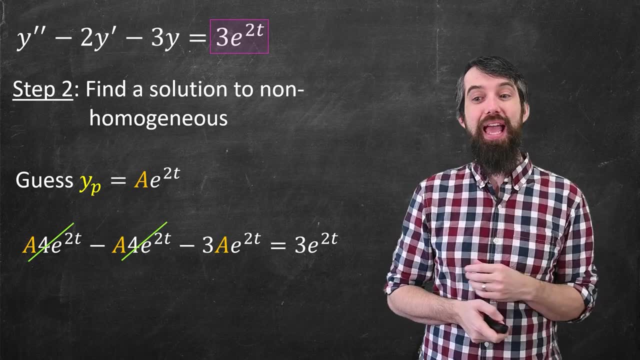 4a and a minus 4a times e to the 2t, Those cancel. That leaves me with minus 3a equals 2,, 3,, and both multiplied by e to the 2t. Well, if that's the case, then a has to be equal to minus 1, and I have a. 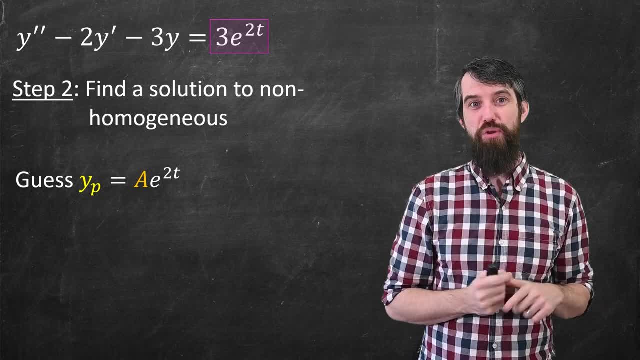 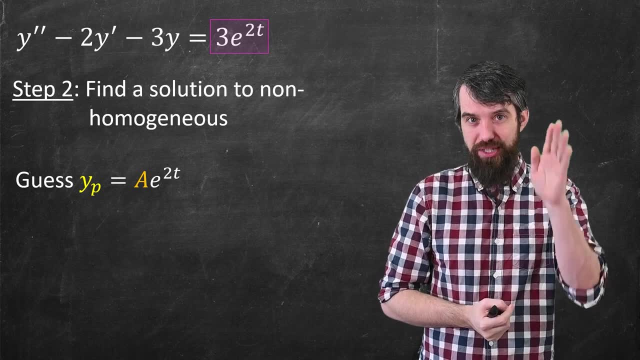 here's my guess: Instead of the 3, I put an undetermined coefficient a, but other than that, I leave the same structure. The e to the 2t is going to be the same. So my guess is that some constant a times e to the 2t. I mean, it's a guess, so let's just plug it in. Well, if I do that. 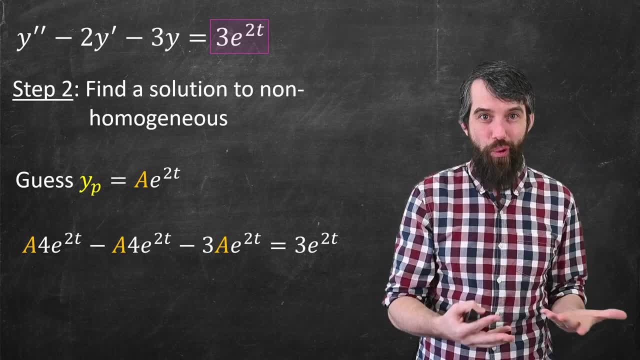 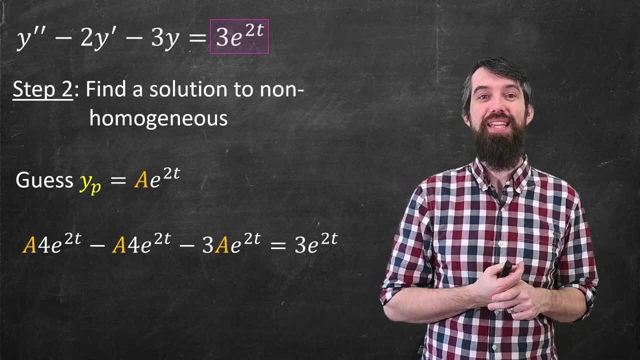 then okay, two derivatives of this is going to give: 2 times 2 is 4 times ae to the 2t, then minus 2 times 2e to the 2t, so now minus 4 times ae to the 2t, and then finally minus 3y minus 3ae to the 2t. 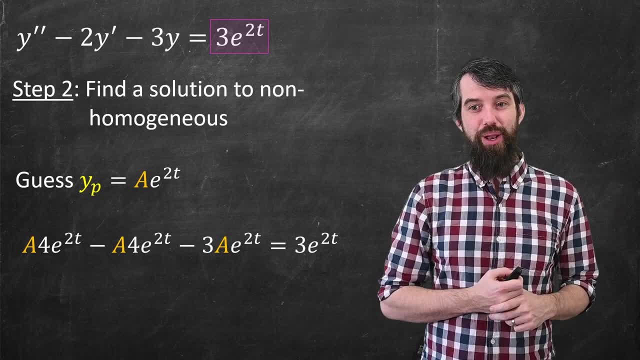 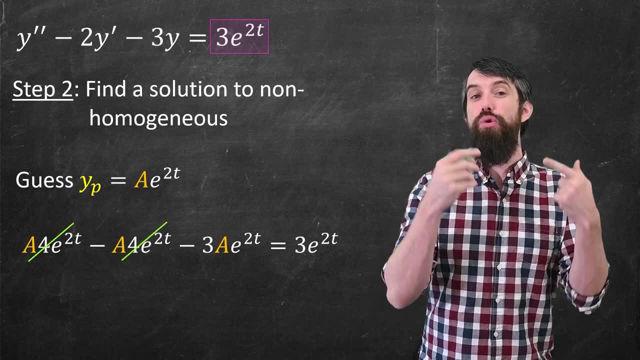 So just a lot of e to the 2t's everywhere. Then observe: well, I have a plus 4a and a minus 4a times e to the 2t. Those cancel. That leaves me with minus 3a equals 2,, 3, and both multiplied. 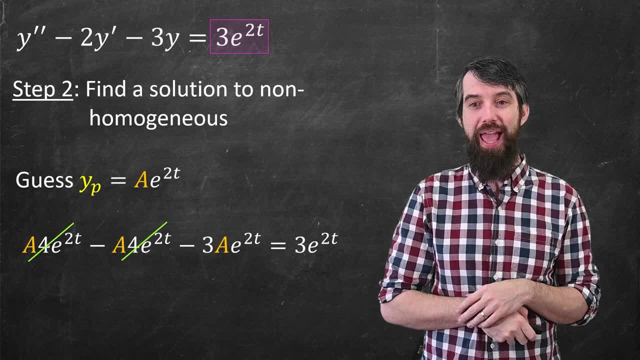 by e to the 2t. Well, if that's the case, then a has to be equal to minus 1, and I have a value for it. now. My particular solution is negative 1 times e to the 2t. 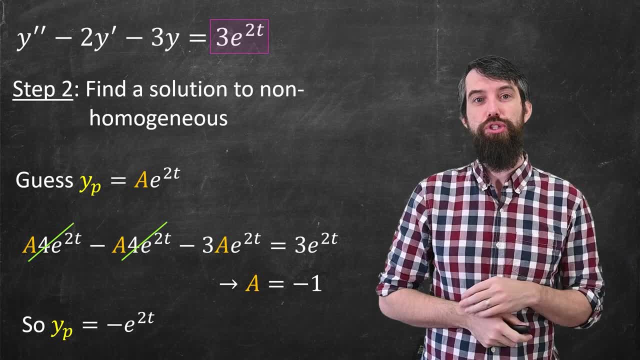 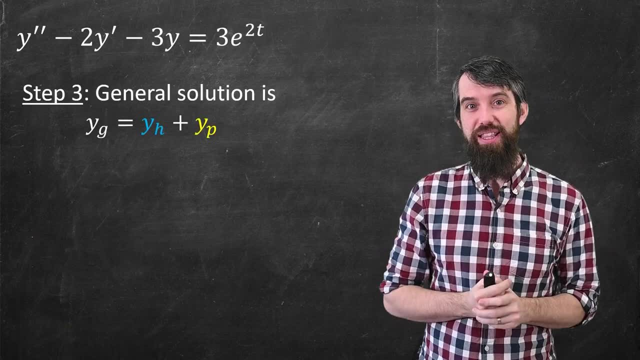 This is a solution. It's not the general solution, but it is a solution. So then, finally, the most important part, step number three: How do I put them together? Well, the general solution to this is the general solution to the homogeneous, plus the one solution you found to the particular. 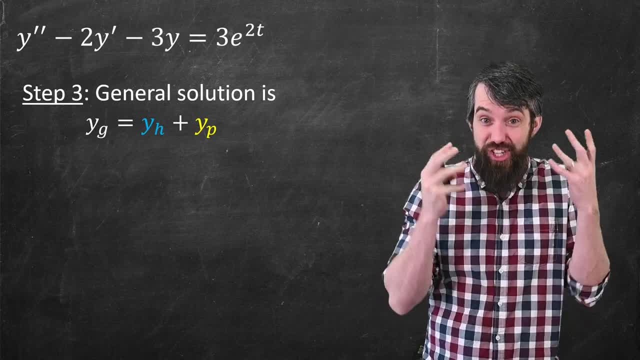 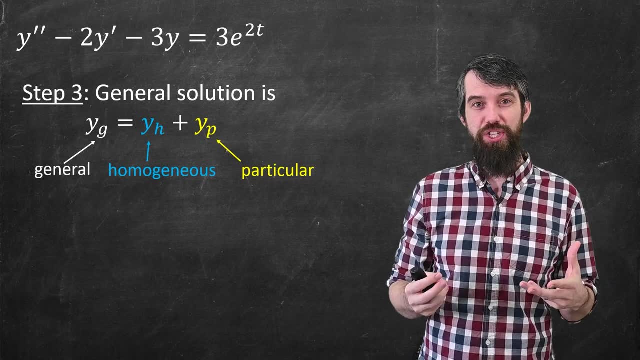 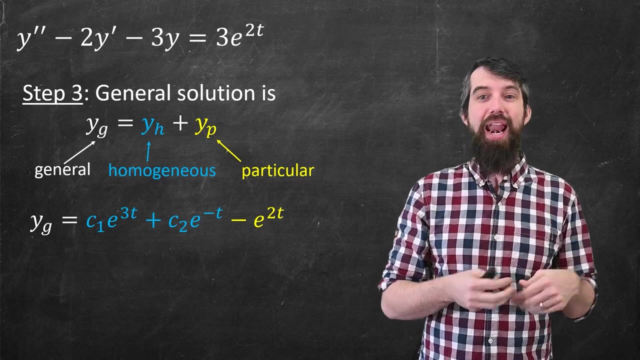 So all sorts of subscripts, characters, let's remind ourselves yg means the general solution, yh the solution to the homogeneous and yp the particular solution, aka the solution to the non-homogeneous. So in my case, I have my homogeneous, that was, the c1e to the 3t and c2e to the minus t, and I have my particular. 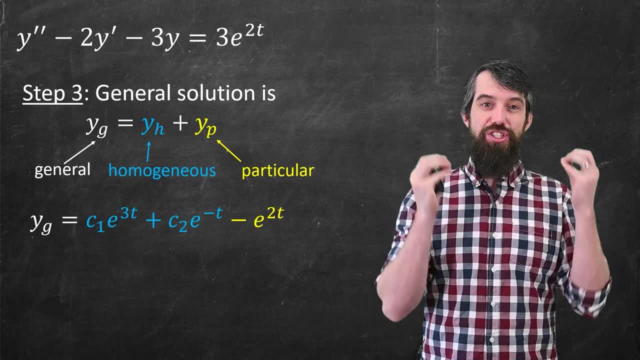 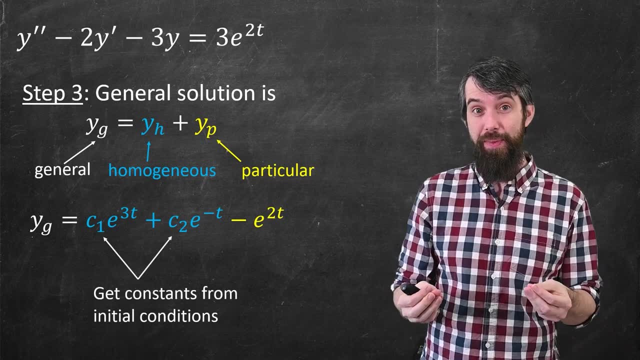 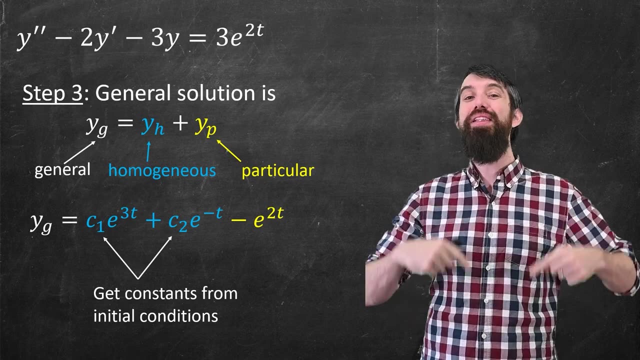 which was negative e to the 2t. That's my general solution. If I had initial conditions, I could plug in and evaluate the c1 and the c2.. Note, by the way, that the order here matters. So you have to form your general, which was your homogeneous, and your particular, and only then. 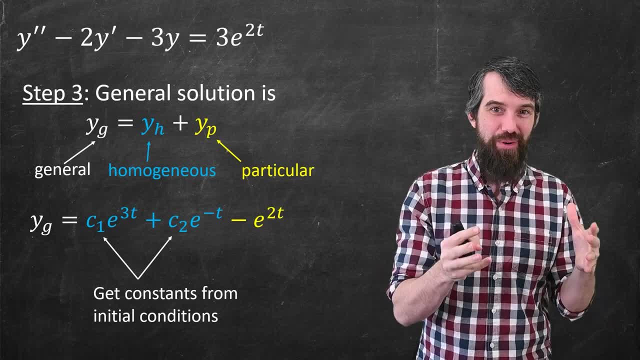 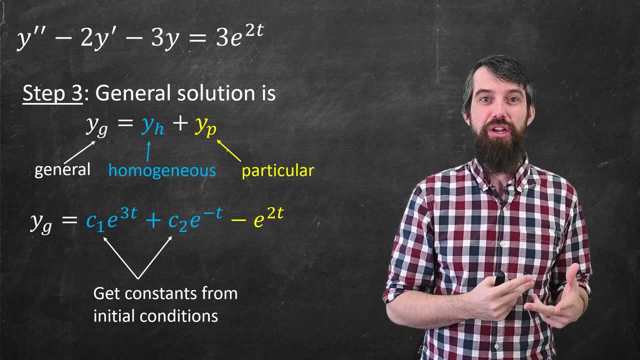 solve for the coefficients. I've noticed in the past students often get the homogeneous. they solve for the coefficients first and only then add for the particular. That order doesn't work out. The second observation here is: just note where the constants are coming from. 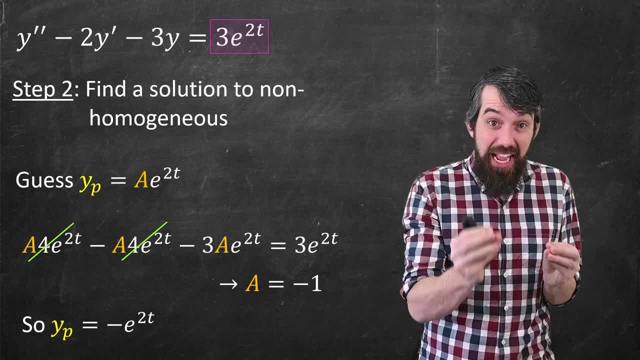 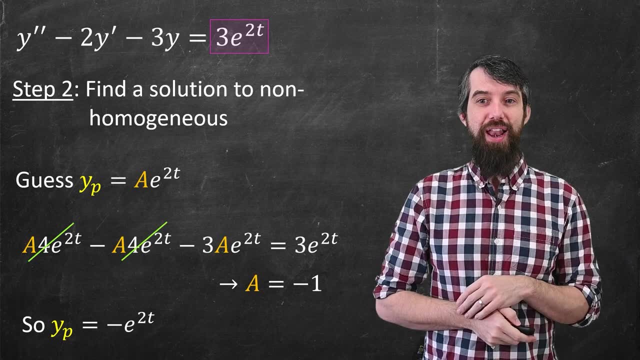 value for it. now, My particular solution is negative 1 times e to the 2t. This is a solution. It's not the general solution, but it is a solution. So then, finally, the most important part, step number three: how do I put them together? Well, the general solution to this. 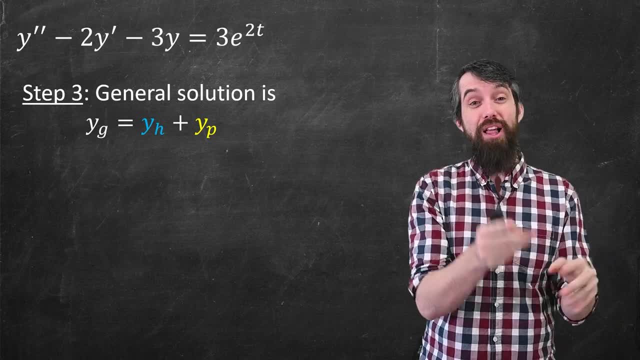 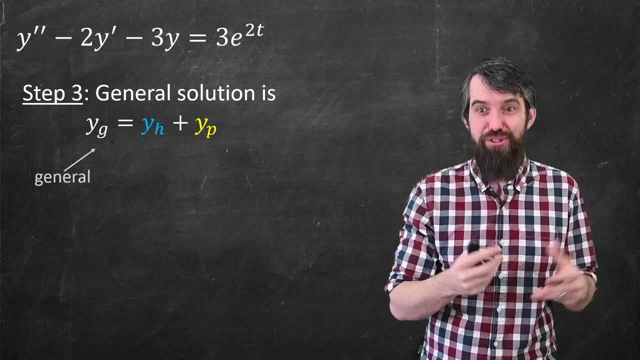 is the general solution to the homogeneous, plus the one solution you found to the particular. So all sorts of subscripts, characters, let's remind ourselves, yg means the general solution, yh the solution to the homogeneous, and yp the particular solution, aka the solution to the. 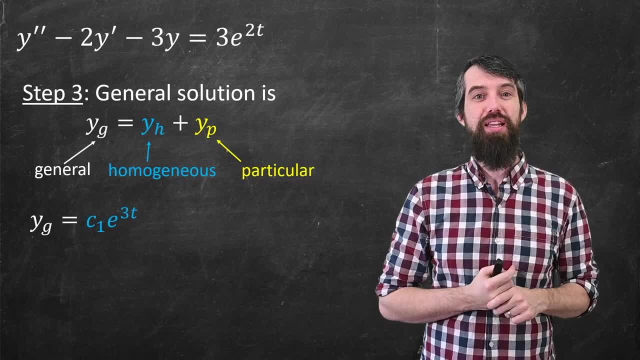 non-homogeneous. So in my case I have my homogeneous, That was the c1 e to the 3t and c2 e to the minus t, and I have my particular, which was negative e to the 2t. 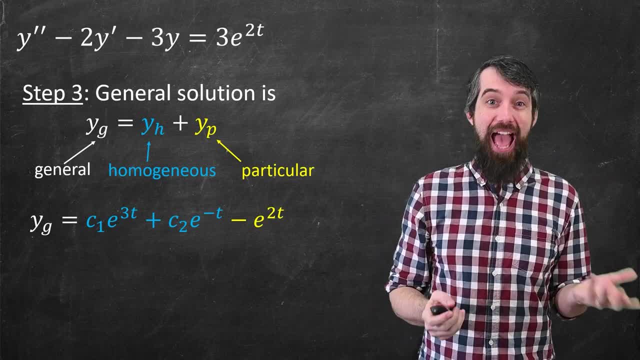 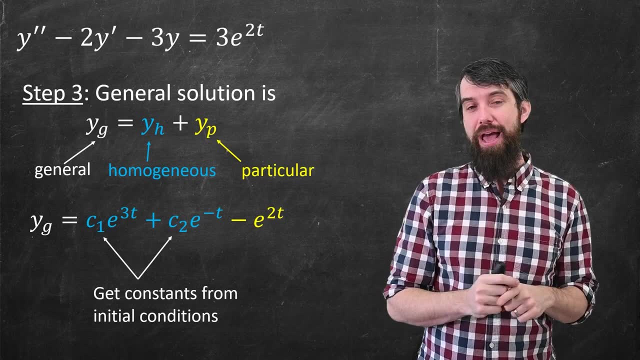 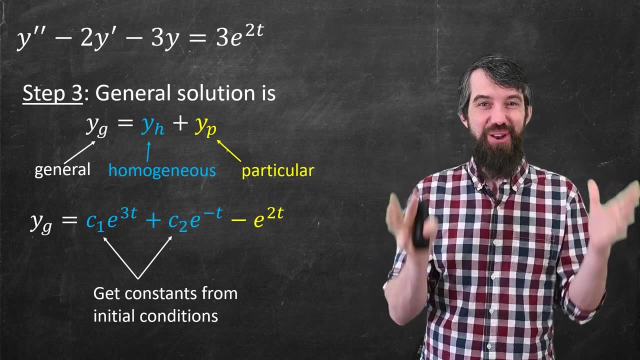 That's my general solution. If I had initial conditions, I could plug in and evaluate the c1 and the c2.. Note, by the way, that the order here matters. So you have to form your general, which was your homogeneous, and your particular, and only then solve for the coefficients I've 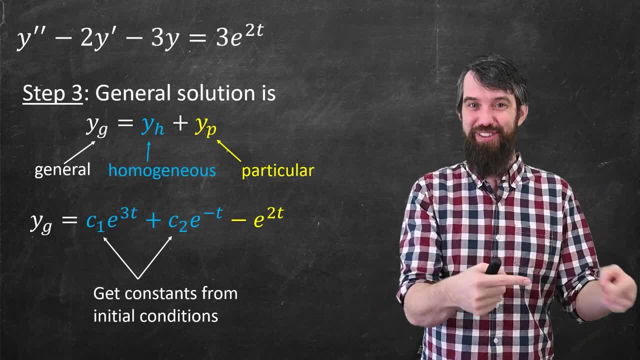 noticed in the past, students often get the homogeneous. they solve for the coefficients first and only then add the non-homogeneous. So I have to form my general, which was your homogeneous, and for the particular. that order doesn't work out. The second observation here is: 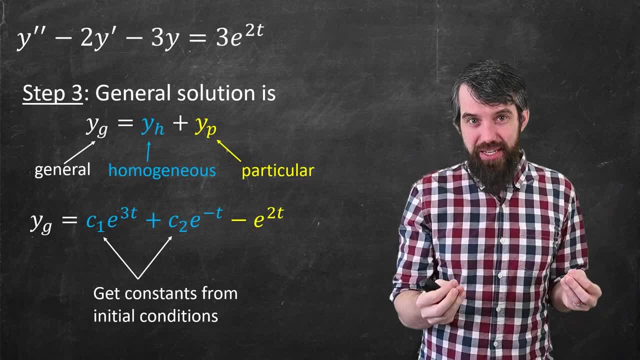 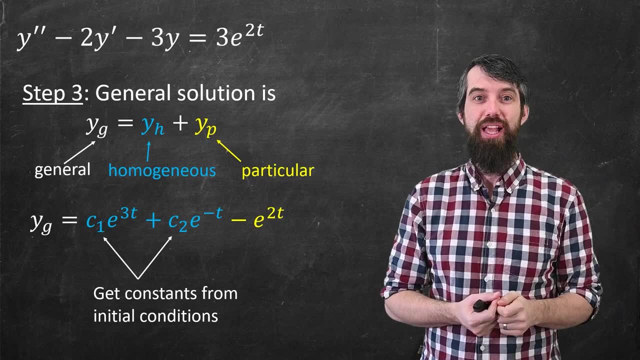 just note where the constants are coming from. The constants are part of the solution to the homogeneous, but the particular, just any one particular one that works. That's why we call it a particular solution. There's no constants in the particular part. Okay, so that's the. 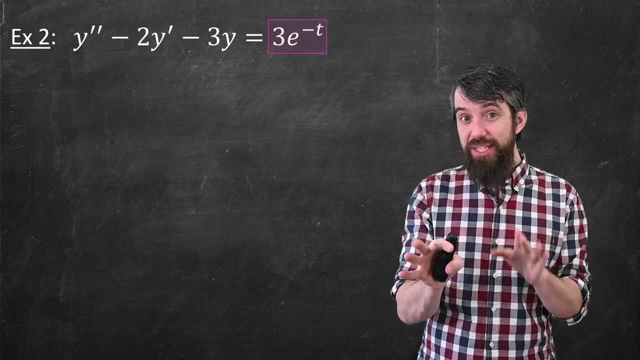 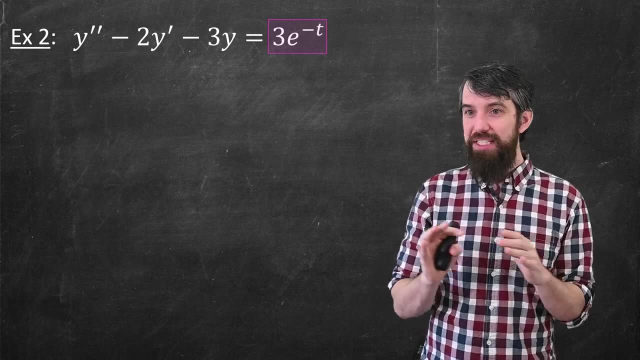 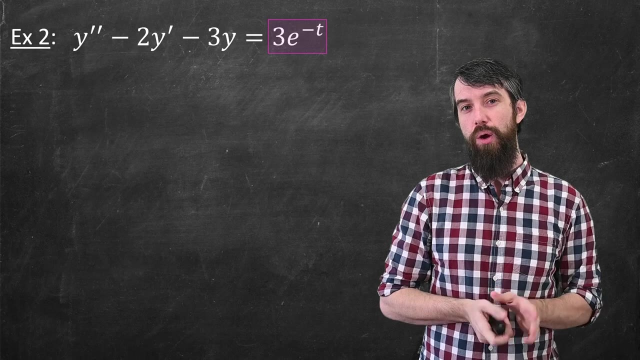 methodology. Let's do one more example. This example is almost the same as the first example. The left-hand side, the constant coefficient part, is identical. The right side is almost the same, except it's 3e to the Minus t, now Not 2t as it was in the previous example. Why does this matter? Well, I mean. 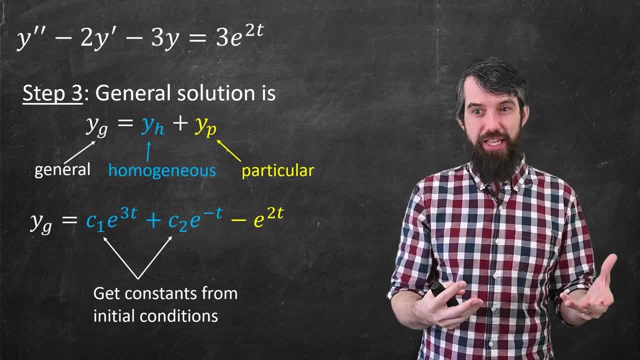 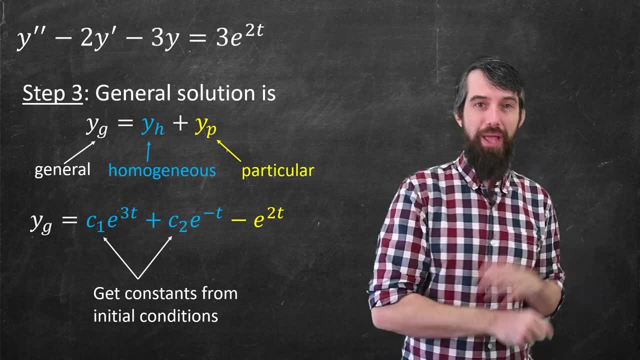 The constants are part of the solution to the homogeneous, but the particular, just any one particular one that works. That's why we call it a particular solution. There's no constants in the particular part. Okay, so that's the methodology. Let's do one more example. This example is almost. 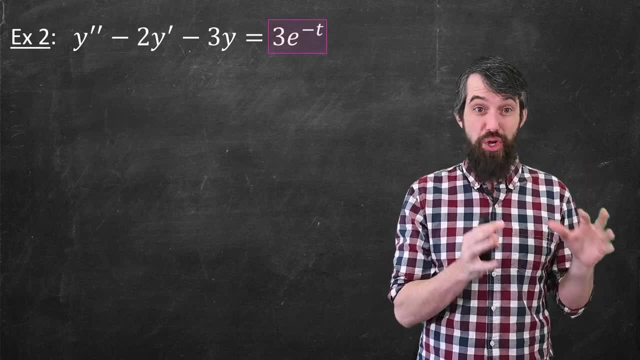 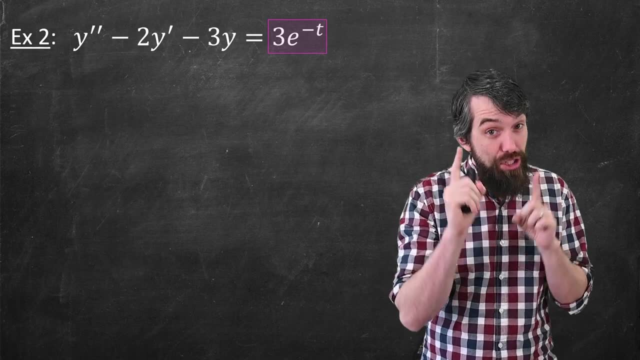 the same as the first example. The left-hand side, the constant coefficient part is identical. The right side is almost the same. The left-hand side is almost the same. The right side is almost the same, except it's 3e to the minus t now, not 2t as it was in the previous example. Why does this? 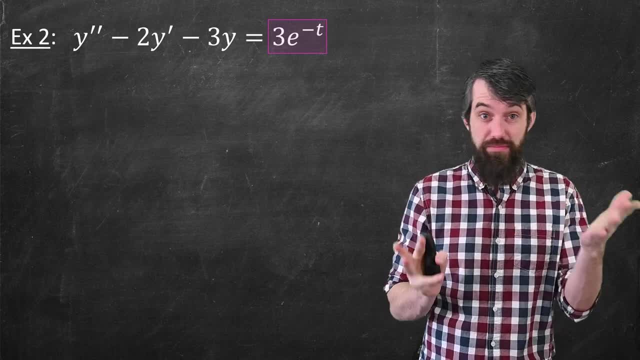 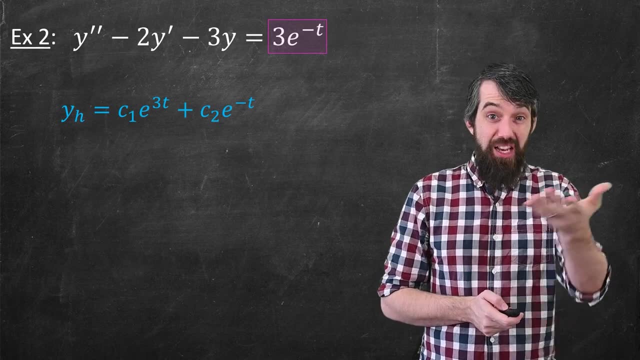 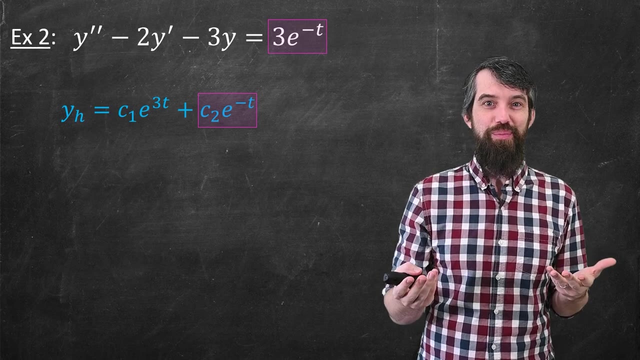 matter. Well, I mean, the homogeneous hasn't changed. We can just quote that one again. But now, if I look at this, you see the e to the minus t, that's the non-homogeneity. The e to the minus t is also there in the solution to the homogeneous system. So a guess of the form. 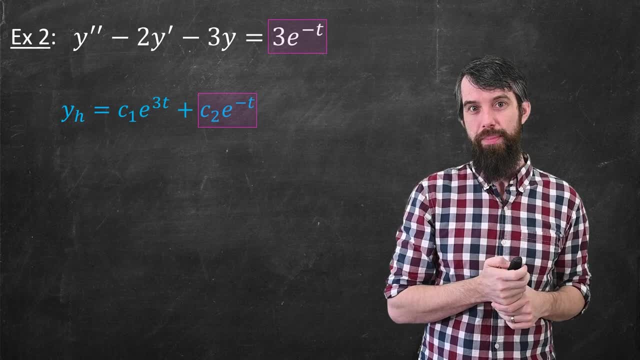 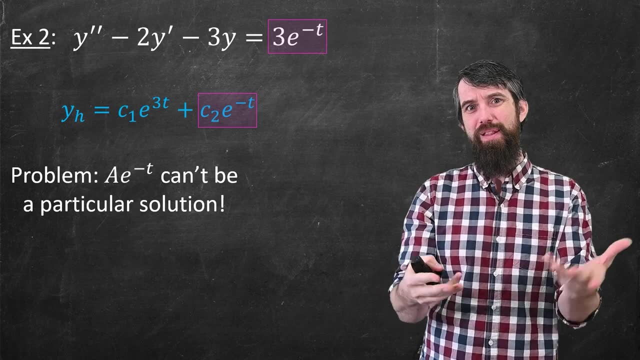 a constant times, e to the minus t cannot work. It cannot work because e to the minus t is a homogeneous solution That would add up to zero. So what can we do? Well, we can do a very analogous trick that we did when we had repeated roots to constant. 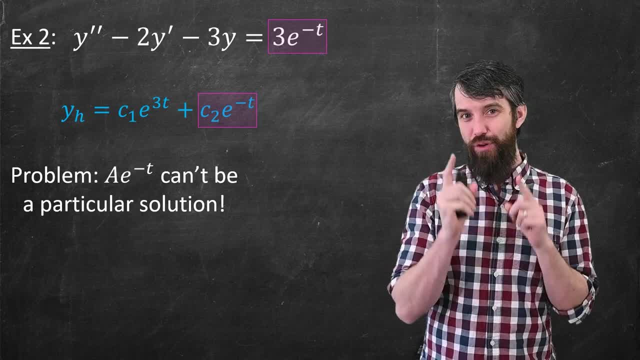 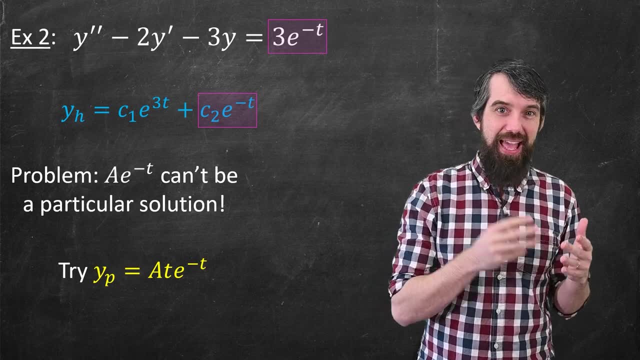 coefficients equations a little while ago. What I'm going to do is, for my yp, I'm going to guess a times t: e to the minus t. Basically, what I've done here is I said well, a, e to the minus t. 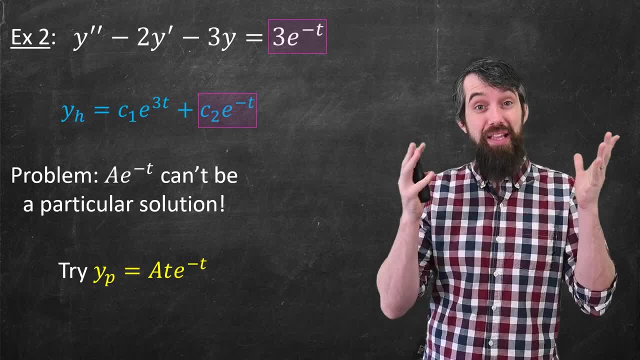 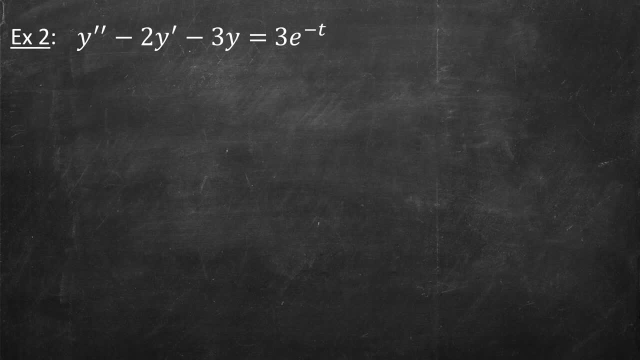 can't work, but if I multiply by one more t out the front, maybe this will work. Okay, well, it's just a guess. right, Could be good, could be bad. Let's plug it in. See, I'm going to have to step away here because this will take a little bit of writing. 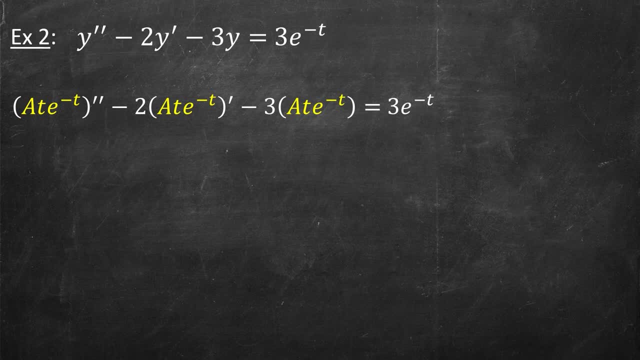 But what I'm going to do is I'm just going to plug in a t e to the minus t. everywhere there's a y. We've got a single derivative and a double derivative. This is going to involve some product rules, So I'm going to step away to give myself a little bit of space here. 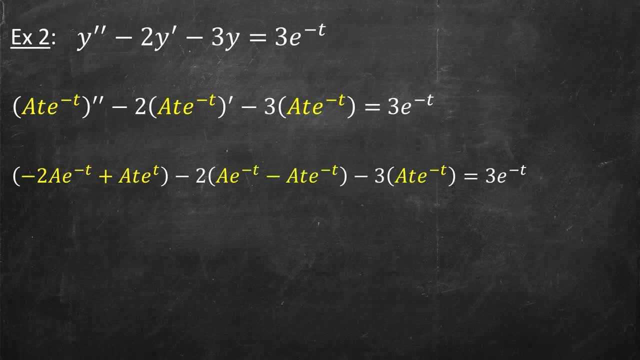 But if I execute those product rules, then I would get well, this long messy expression. You can check it if you wish. What I do want to note, though, is that, if I look at all the terms that are of the form t e to the t, well, I have an a. 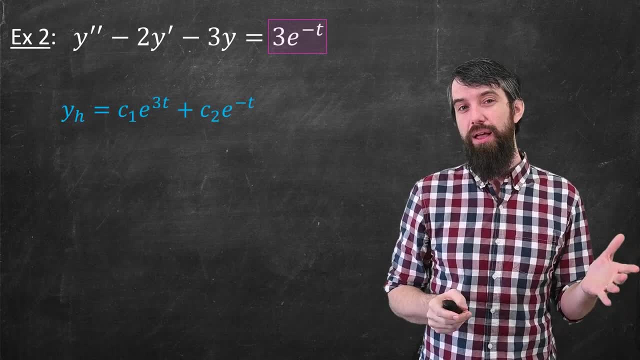 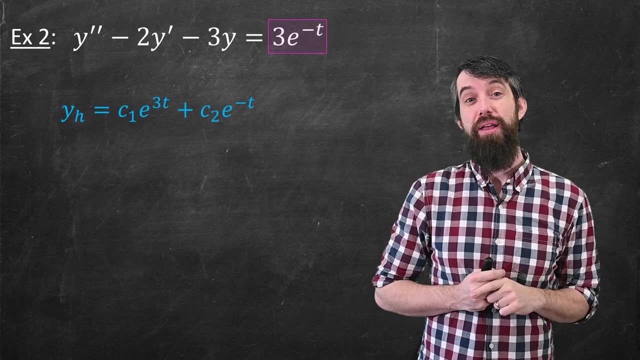 the homogeneous hasn't changed. We can just quote that one again. But now if I look at this, you see the e to the minus t, that's the non-homogeneity. The e to the minus t is also there in the solution to the homogeneous system. So a guess of the form: a constant times e to the. 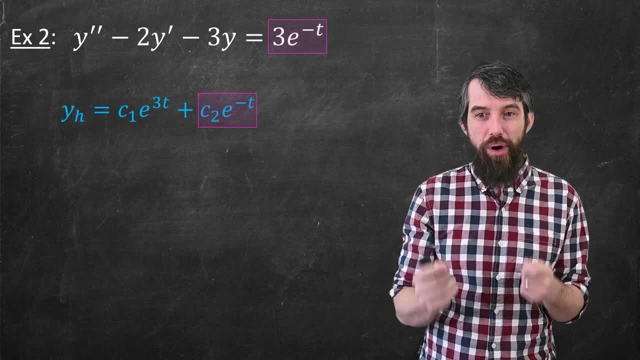 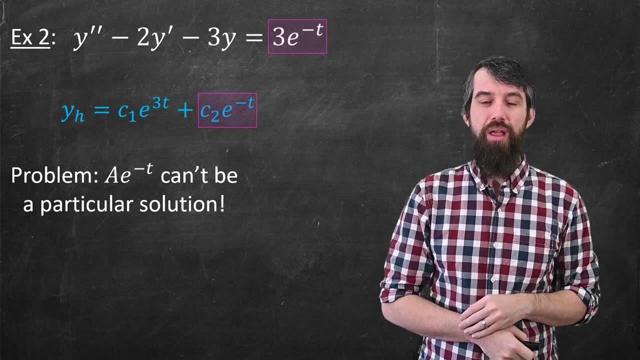 minus t cannot work. It cannot work because e to the minus t is a homogeneous, So it's not a homogeneous solution. That would add up to zero. So what can we do? Well, we can do a very analogous trick that we did when we had repeated roots to constant coefficients. equations a little. 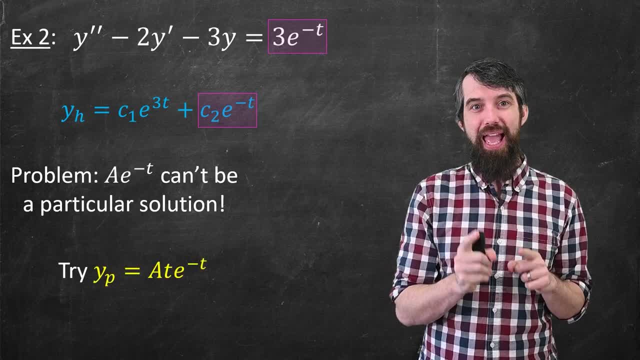 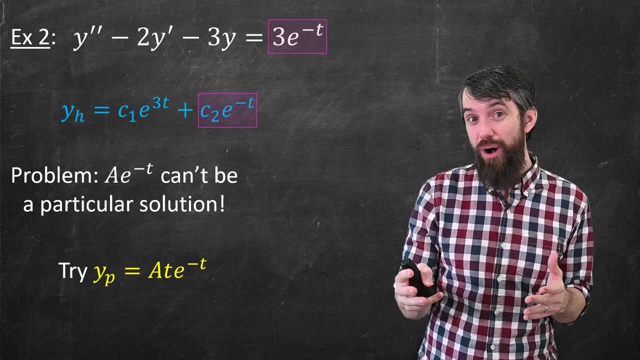 while ago. What I'm going to do is for my yp, I'm going to guess a times t e to the minus t. Basically, what I've done here is: I said well, a e to the minus t can't work, but if I multiply, 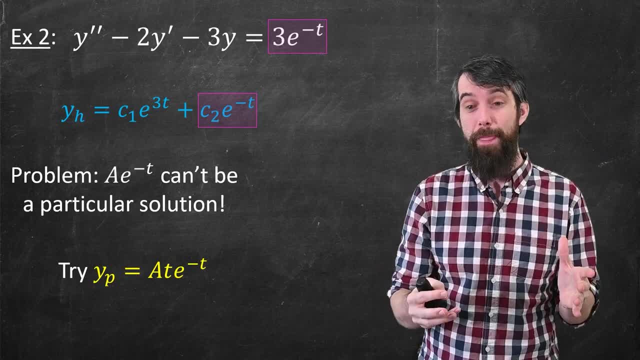 by one more t out the front. maybe this will work, Okay, well, it's just a guess, right? Could be good, could be bad. Let's plug it in and see I'm going to have to step away here and I'm going to. 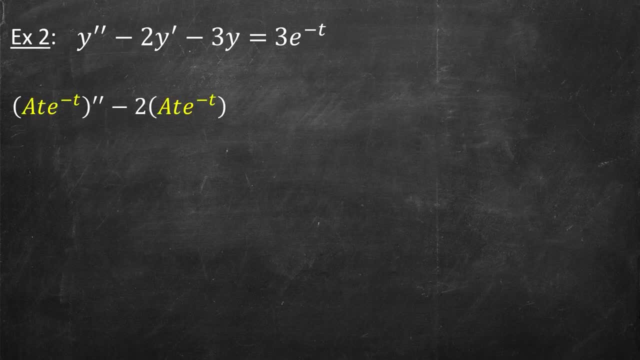 because this will take a little bit of writing. But what I'm going to do is I'm just going to plug in a t e to the minus t. everywhere there's a y. We've got a single derivative and a double derivative. This is going to involve some product rules, so I'm going to step away to give myself a. 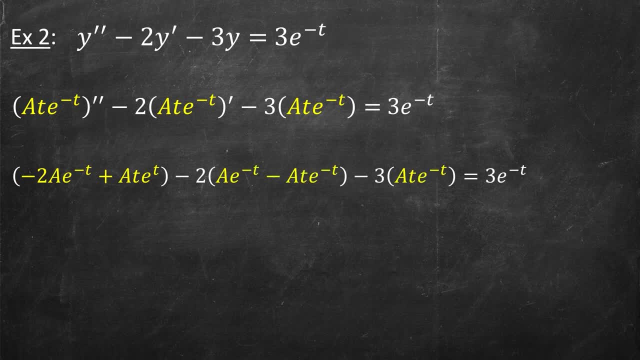 little bit of space here, But if I execute those product rules, then I would get well, this long messy expression. You can check it if you wish. What I do want to note, though, is that, if I look at all the terms that are of the form t, e to the t, well, I have an a, I have a plus two. 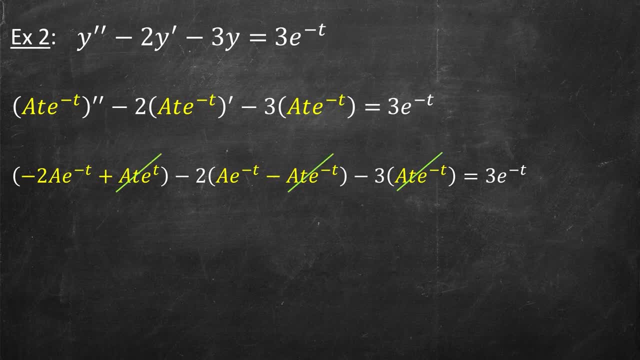 a, and then I have a minus three a, which cancel. So those three terms all cancel. That leaves you with: well, if you count them up, minus four, a e to the minus t is equal to three e to the minus t. 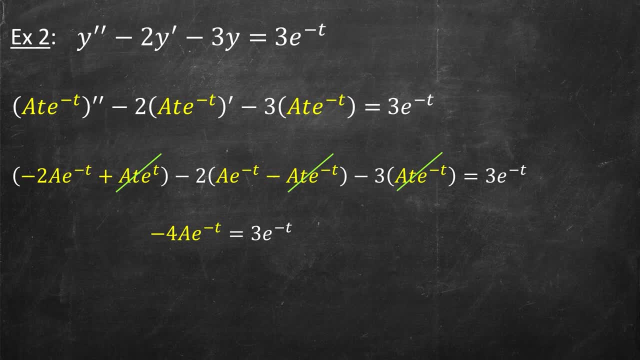 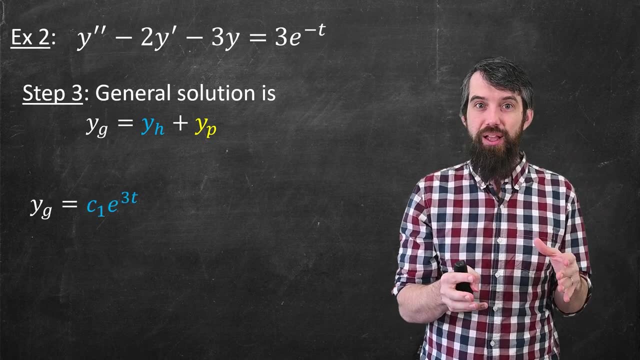 which is the right-hand side. Okay, so then what does that mean? a has to be a, has to be negative three quarters, and thus I can state what my general solution is. My general solution was the homogeneous plus the particular. The particular is minus three quarters t e to the minus t, So the 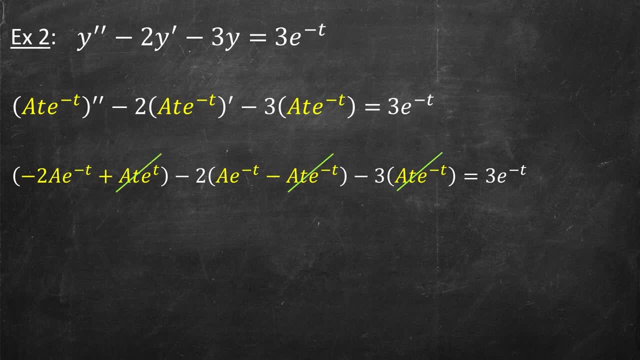 I have a plus 2 a and then I have a minus 3 a, which cancel. So those three terms all cancel. That leaves you with: well, if you count them up, minus 4 a e to the minus t is equal to 3. 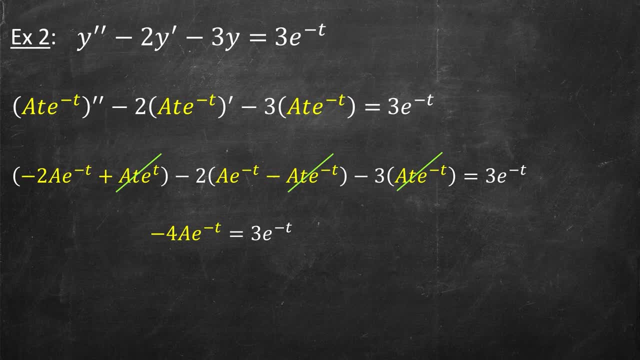 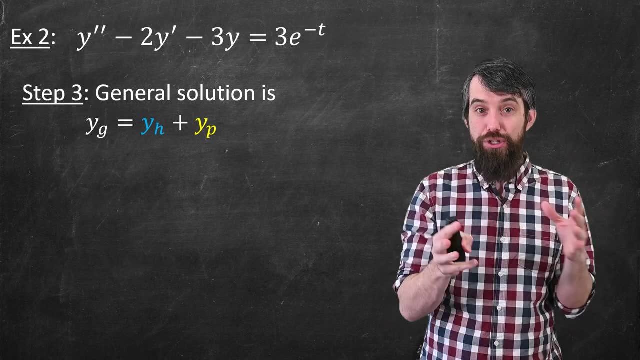 e to the minus t, which is the right-hand side. Okay, so then, what does that mean? a has to be a, has to be negative three quarters, And thus I can state what my general solution is. My general solution was the homogeneous plus the particular. The particular is minus three quarters. t? e to the. 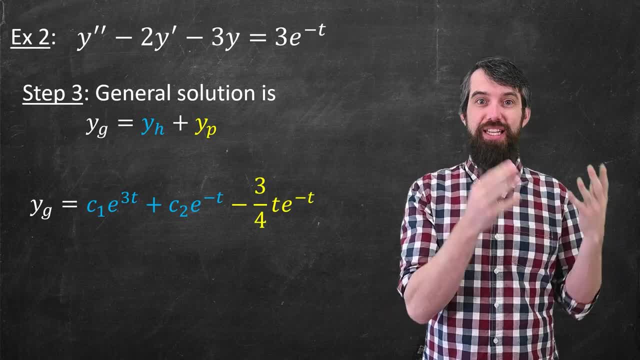 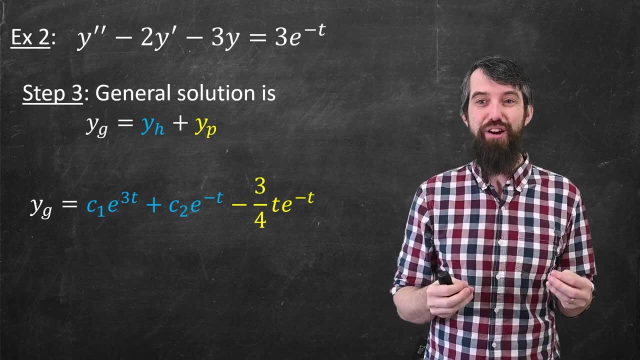 minus t. So the mess is the same. solve the homogeneous in general and then guess just some particular one and then add them together. by our theory, The only difference was you had to be a little bit more careful about your y particular, just to make sure it didn't overlap. 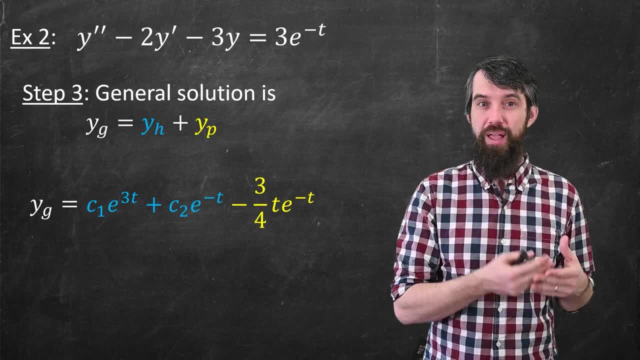 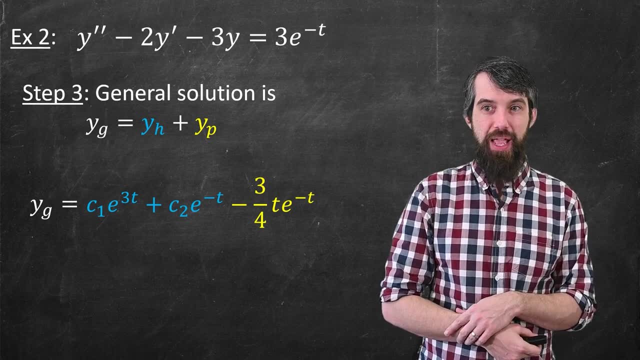 with one of the solutions for the homogeneous equation. So then we turn to the question of: I mean, what kind of guesses should you do in general? So let me put up a little bit of a chart here. So the left column, I have different types of non-homogeneities, the things that could show. 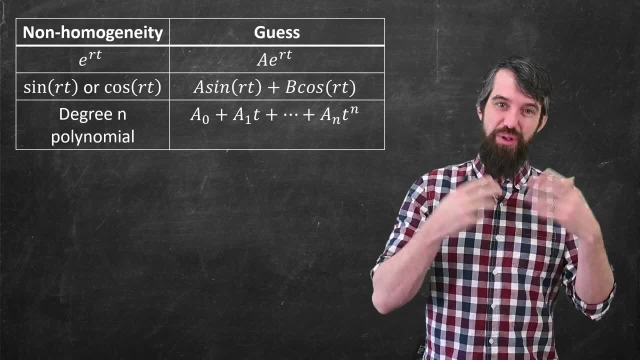 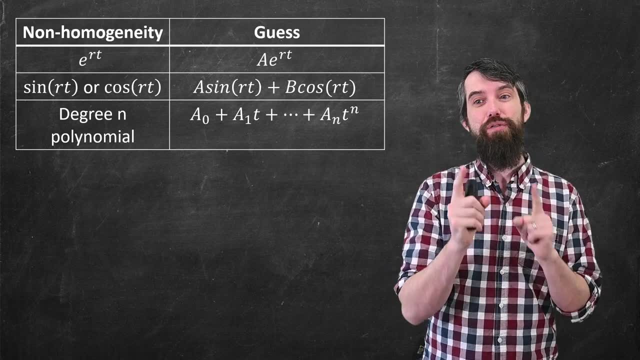 up on the right-hand side of your equation. So if you look at this you're going to see that the side of your equation a bit confusingly. So, for example, you have exponentials or polynomials or sine and cosine terms And in the right column I've told you what you should guess for your y. 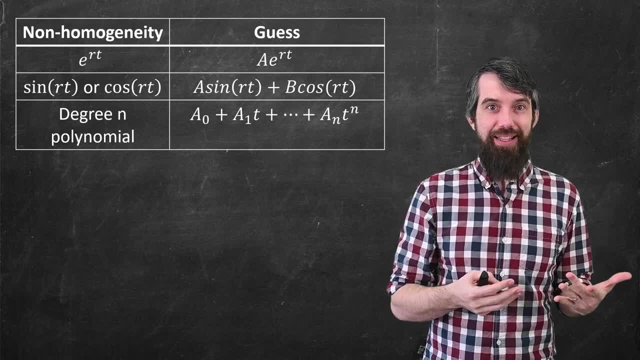 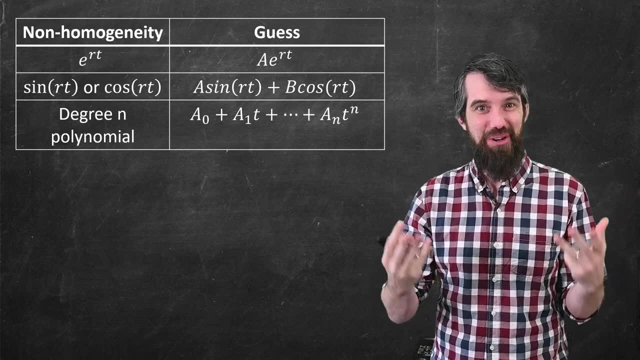 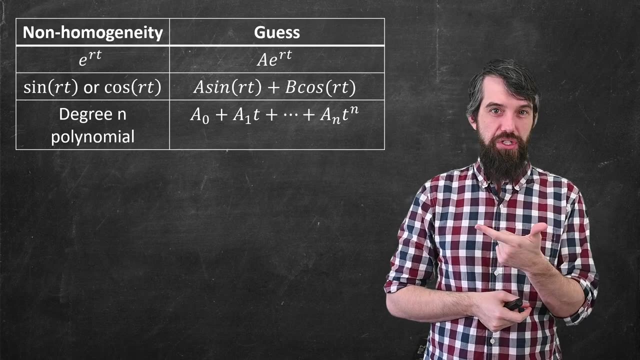 particular. So, for instance, we saw, if it was exponential, guess an exponential of the same form: a e to the rt, where a is an undetermined coefficient. in the method of undetermined coefficients, If it's a sine term or if it's a cos term, well, you can guess a sine and a cos of. 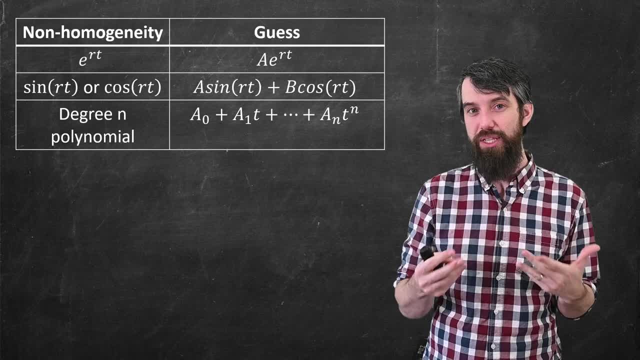 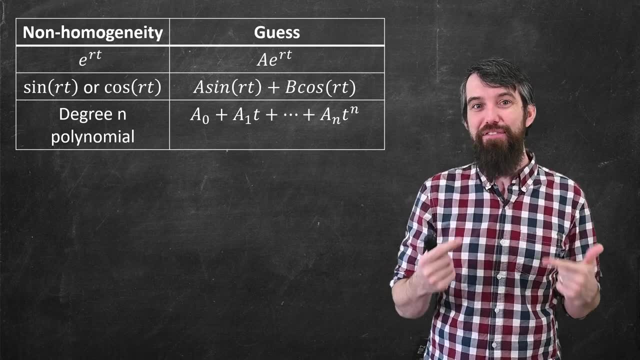 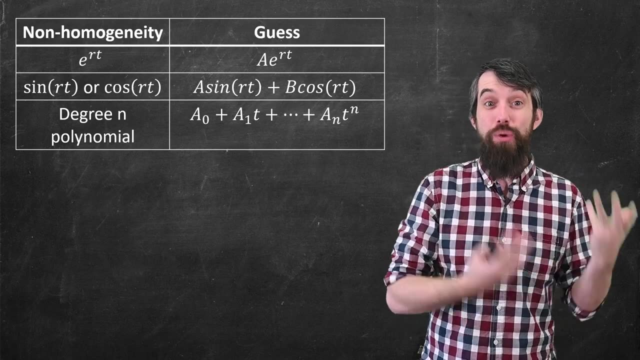 the same frequency like sine rt. you guess sine rt. But here's the trick: You have to have a sine of rt plus b cosine of rt, even if your left-hand side only had one of those two terms. The idea is that derivative of sine is cosine, derivative of cosine is sine, So you need to have both sines. 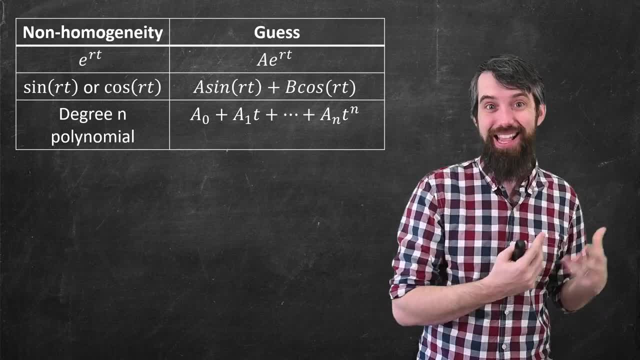 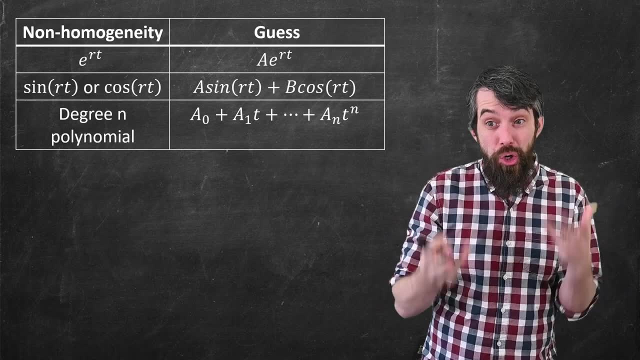 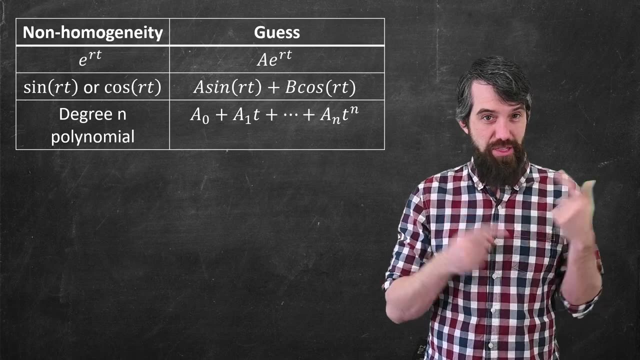 and cosines in your guess, if there's any sines or cosines appearing in the non-homogeneity, And then for a degree n polynomial, like say t squared, you'd guess a degree 2 polynomial, the generic Degree 2 polynomial, a0 plus a1t, all the way up to antvn. And then there's two caveats. The first: 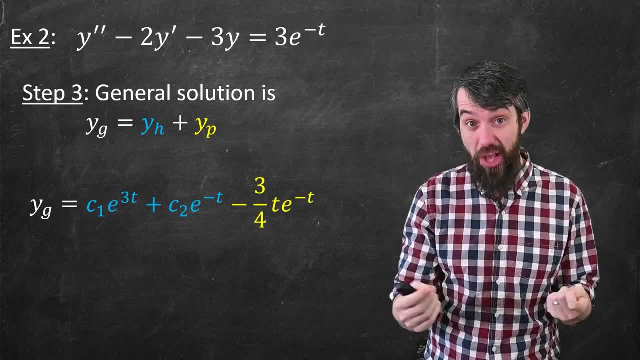 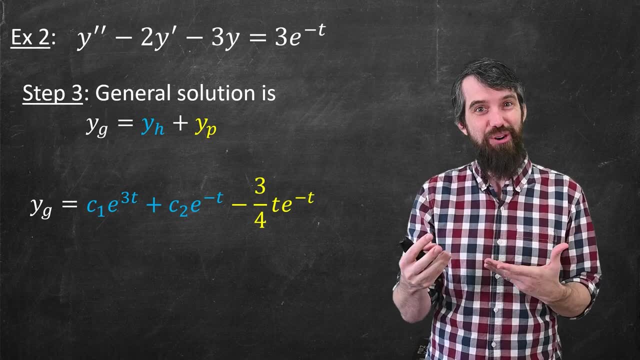 same: Solve the homogeneous in general and then guess just some particular one and then add them together. by our theory, The only difference was you had to be a little bit more careful about your y particular, just to make sure it didn't overlap with one of the solutions for the homogeneous. 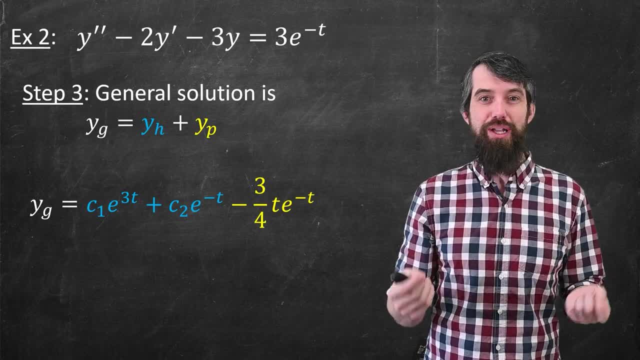 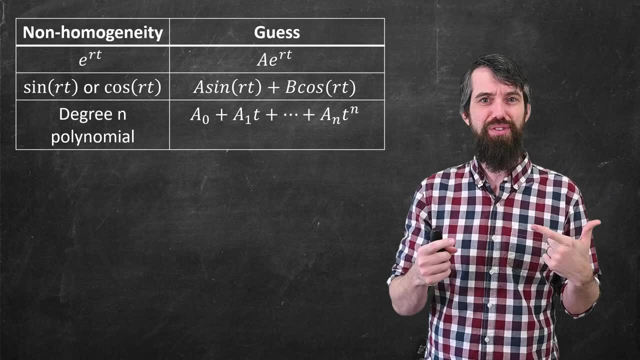 equation. So then we turn to the question of: I mean, what kind of guesses should you do in general? So let me put up a little bit of a chart here. So the left column: I have different types of non-homogeneities, the things that could show up on the right-hand side of your equation a bit. 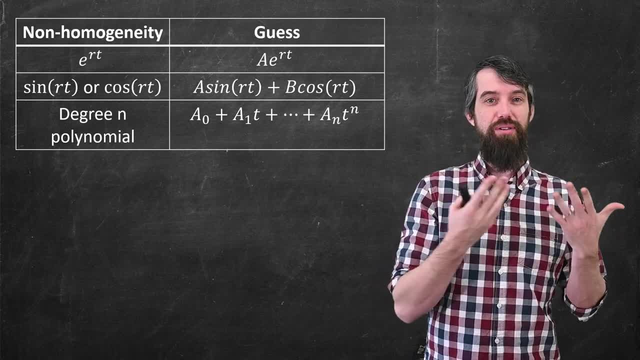 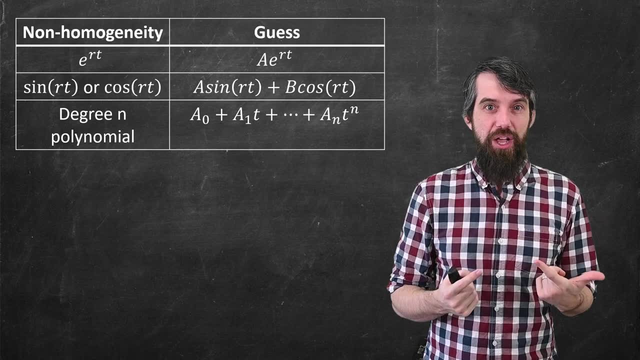 confusingly. So for example, you go exponentials or polynomials or sine and cosine terms, And in the right column I've told you what you should guess for your y particular. So for instance we saw, if it was exponential, guess an. 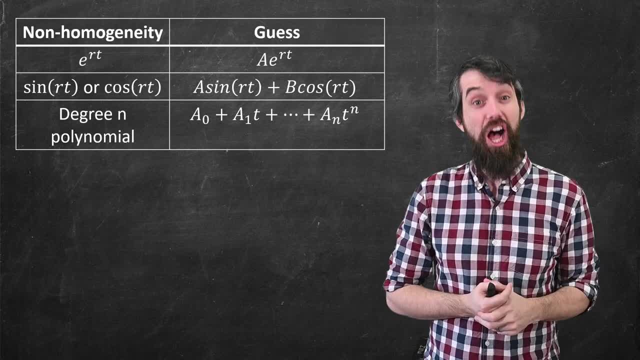 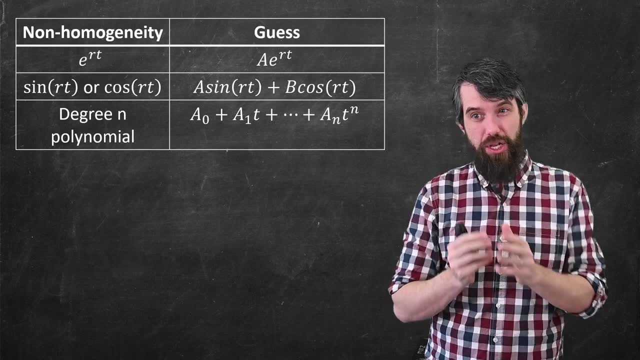 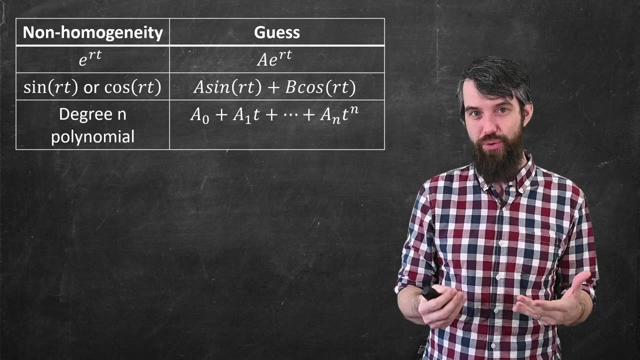 exponential of the same form, a e to the rt, where a is an undetermined coefficients. in the method of undetermined coefficients, If it's a sine term or if it's a cos term, well, you can guess a sine and a cos of the same frequency, like sine rt, you guess sine rt. But here's the trick: You have to. 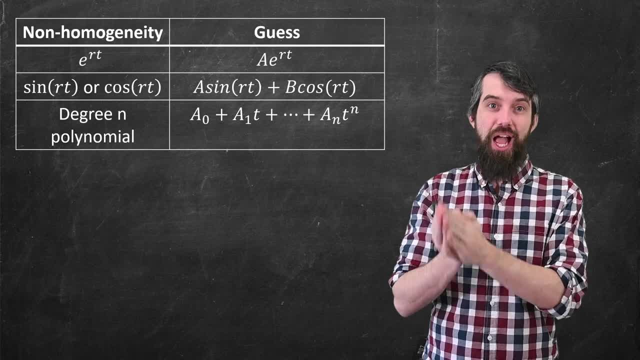 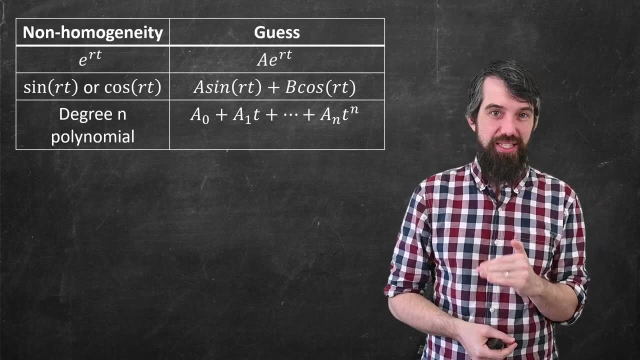 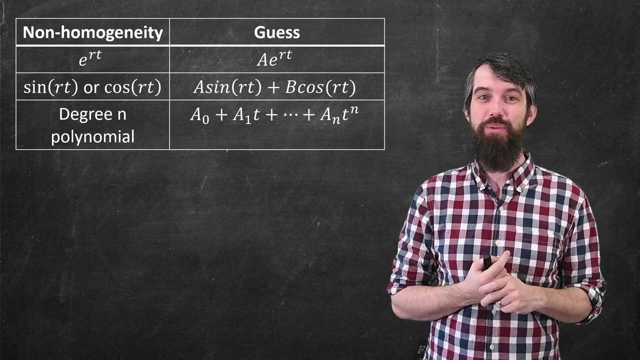 have a sine of rt plus b cosine of rt, even if your left-hand side only had one of those two terms. The idea is that derivative of sine is cosine, derivative of cosine is sine, So you need to have both sines and cosines in your guess if there's any sines or cosines appearing in the non-homogeneity. 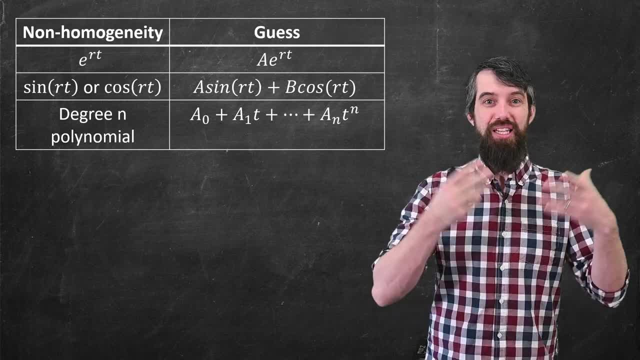 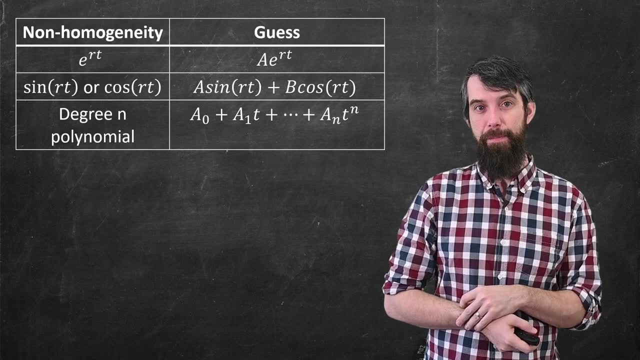 And then for a degree n polynomial like, say, t, squared, you'd guess, a degree two polynomial, the generic degree two polynomial, a zero plus a one t, all the way up to a n, t to the n. And then there's two caveats. The first caveat is what we talked about: You might need to multiply. 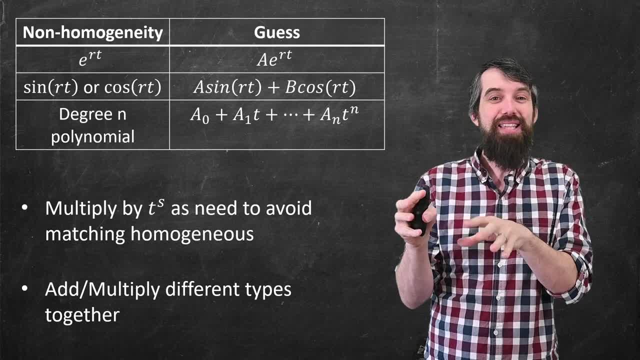 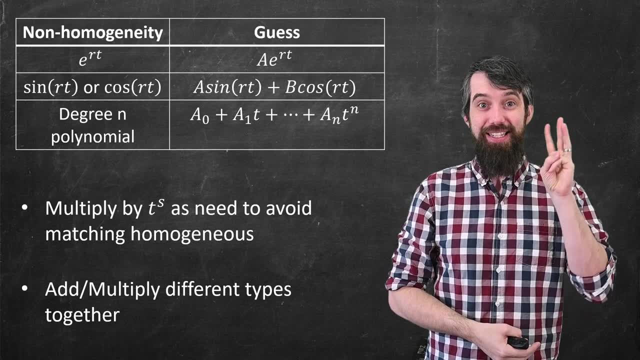 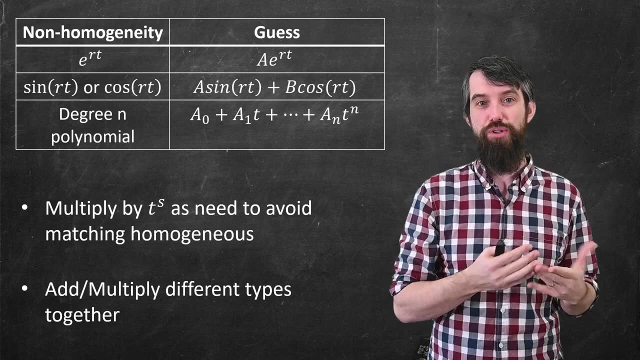 by some t's. If the solution that you get is a matching to the homogeneous, you multiply by t or t squared or t cubed, however many multiplications of t's to a natural number. s is a natural number you need so that the result you get is not a matching to the homogeneous. 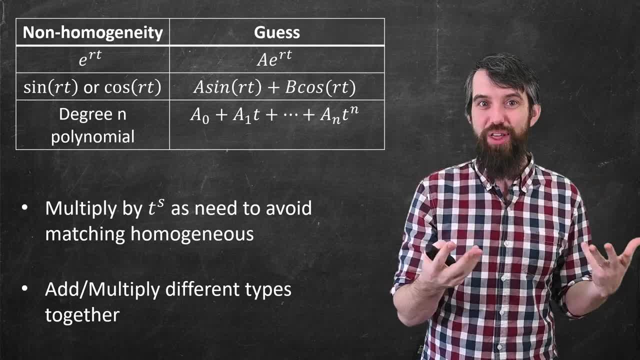 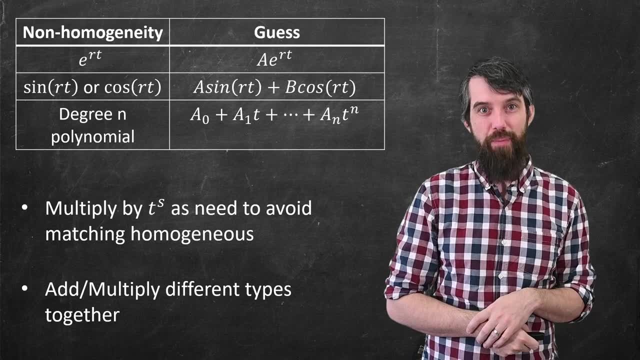 And then the final caveat being that you might have a combination of these, like the sum of them, or a multiplication of them, in which case you add or multiply the guesses as well. So a final illustration of this. I won't do the algebra for it, but I'll tell you what the guess. 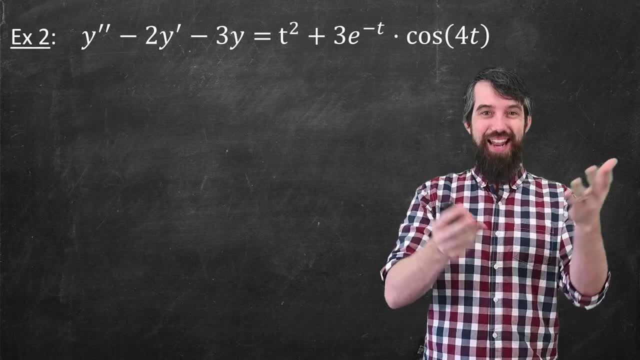 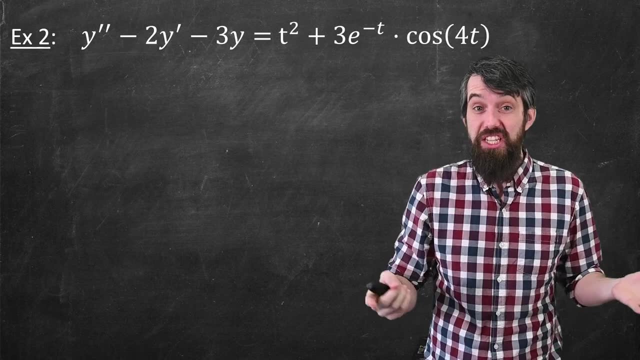 is So same left-hand side, same homogeneous part, but the right-hand side is really messy. now t squared plus three to the minus t times cosine of four t. it's a mess. So my homogeneous, we know what to do there. but what about my particular? So the particular is a bunch of things For the t. 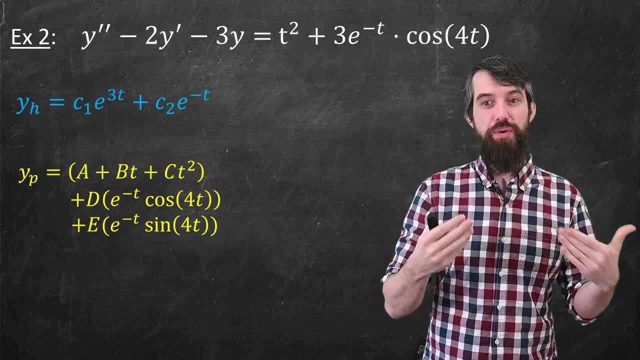 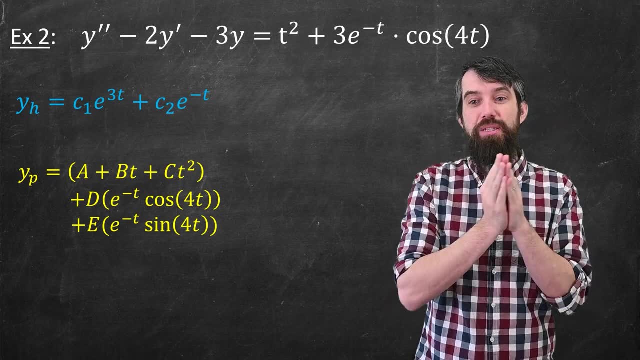 squared, that was a polynomial. So you guess a generic degree two, polynomial. Now note, I'm not guessing c, t squared, I'm guessing a generic degree two, polynomial. So you guess a generic degree two polynomial: a plus b, t plus c, t squared. You got to include all the terms of less degrees than that. 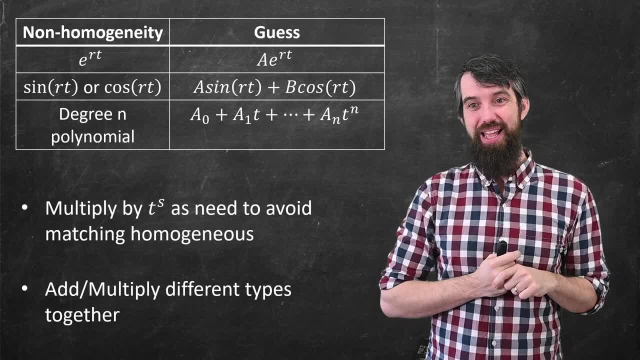 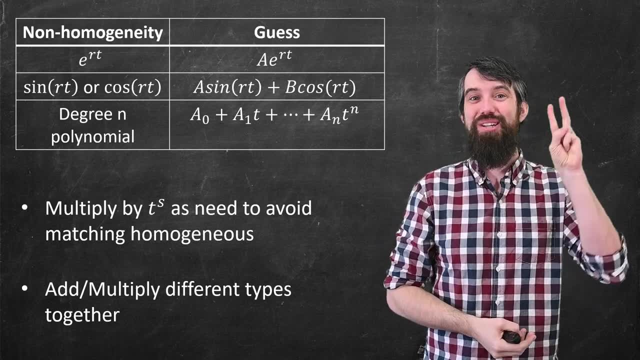 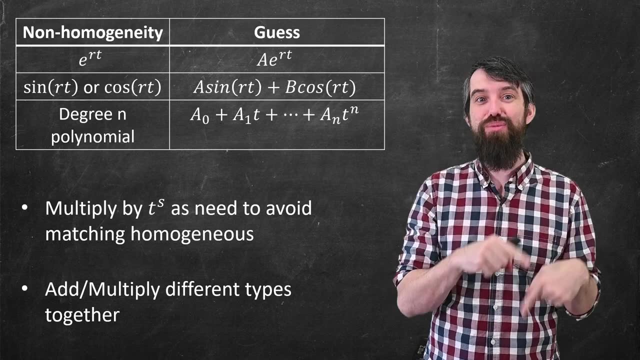 caveat is what we talked about. You might need to multiply by some t's. If the solution that you get is a matching to the homogeneous, you multiply by t or t squared or t cubed. however many multiplications of t's to a natural number- s is a natural number you need so that the result you 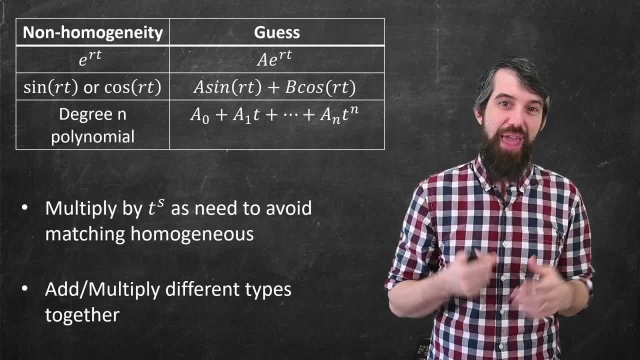 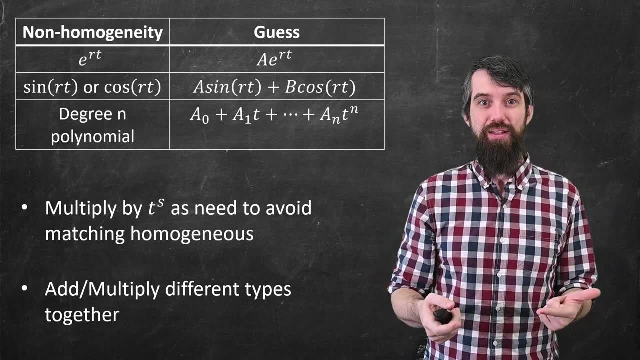 get is not a matching to the homogeneous. And then, the final caveat being that you might have a combination of these, like the sum of them, or a multiplication of them, in which case you add or multiply the guesses as well. So a final illustration of this. I won't do the algebra for. 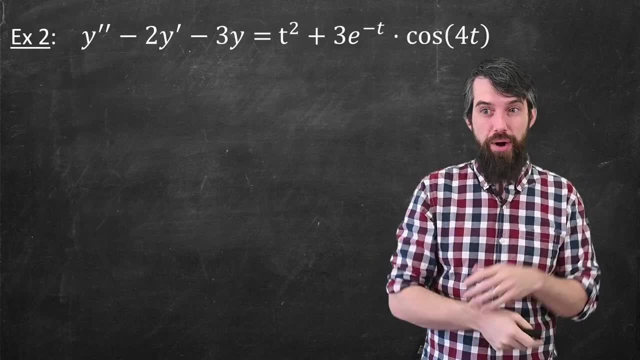 it, but I'll tell you what the guess is. So, same left-hand side, same homogeneous part, but the right-hand side is really messy now. t squared plus 3 to the minus t times cosine of 4t. it's a mess. 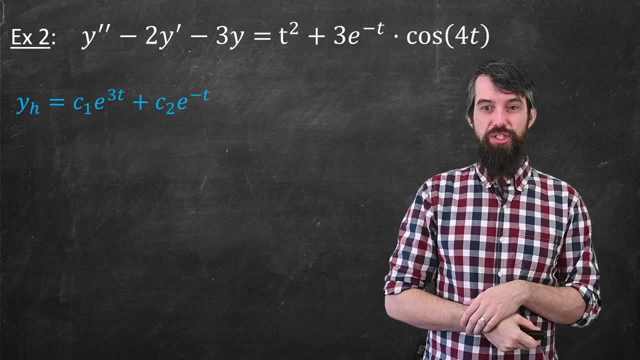 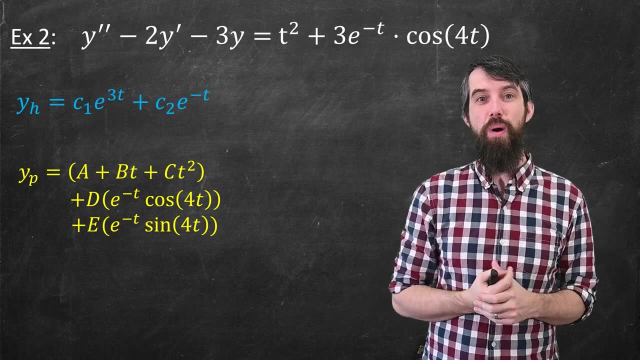 So my homogeneous, we know what to do there. But what about my particular? So the particular is a bunch of things. For the t squared, that was a polynomial, So you guess a generic degree 2 polynomial. So you get a t squared plus 3 to the minus t times cosine of 4t. So you: 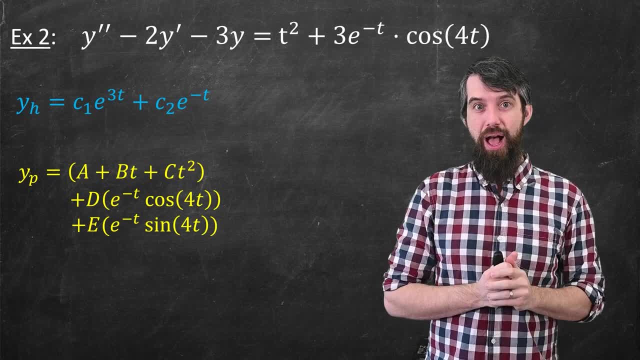 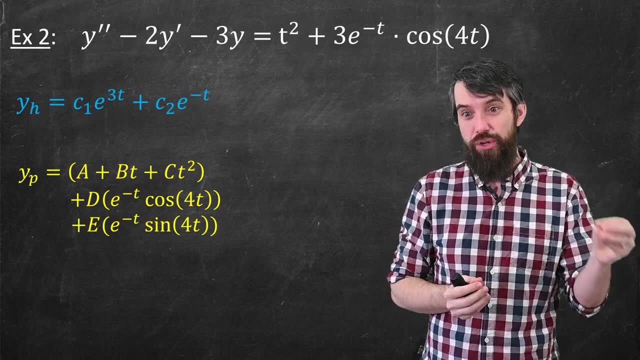 get a t squared plus 3 to the minus 2 polynomial. Now note, I'm not guessing ct squared, I'm guessing a generic degree 2 polynomial, a plus bt, plus ct squared. You got to include all the terms of less degrees than that. Then, for the exponential times, the cosine. we've seen that if there's a 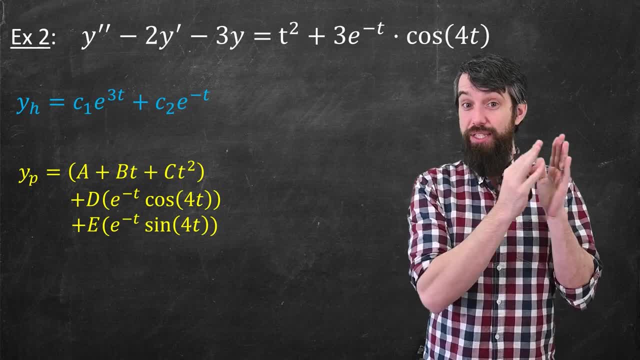 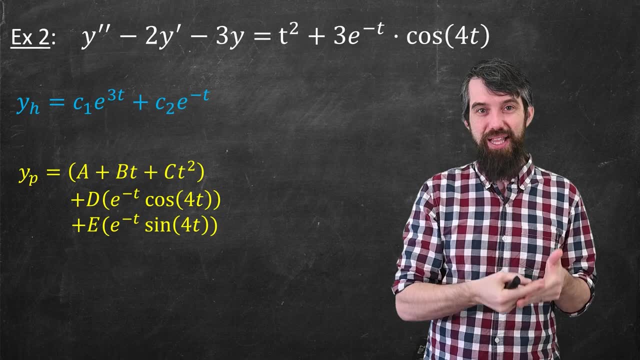 cosine term. you have to have a cosine plus a sine term. So I'll do that: A constant d times the exponential cosine of 4t and then a constant e times the exponential times sine of 4t. You have to have both the cosine and the sine terms. So I'll do that. So I'll do that. 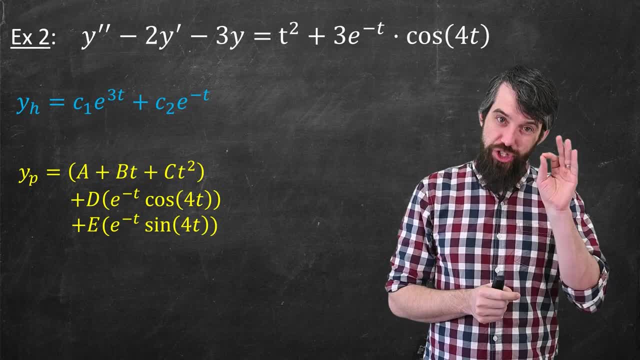 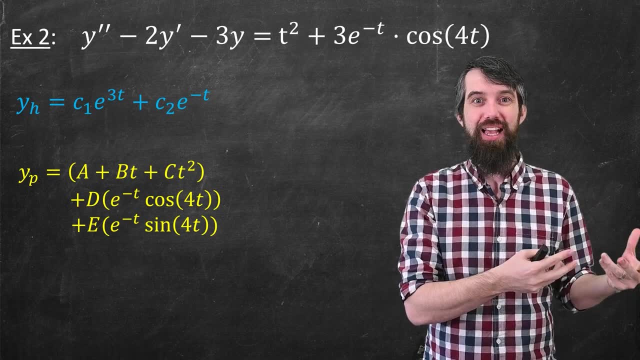 Added together with different coefficients. Final note is that if it was just e to the minus t without the cosine, you would have had to multiply by the extra value of t. So you didn't match the homogeneous, as I did in the previous example. But here e to the minus t times cosine. that is not. 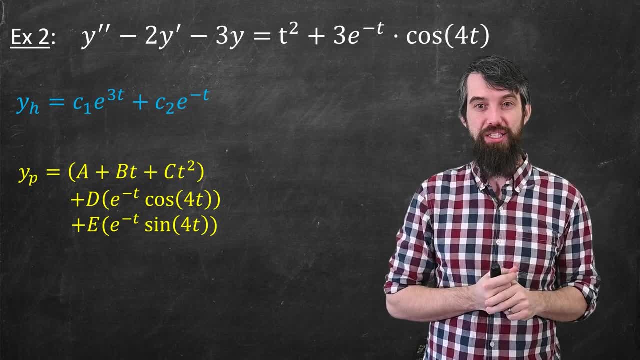 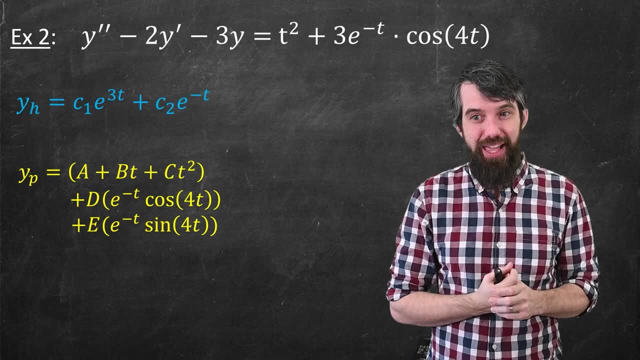 a solution to the homogeneous, And so there's no need to multiply by any extra t. So that would be my guess. Now, if you plug it in, there's going to be five different variables: a, b, c, d and e. 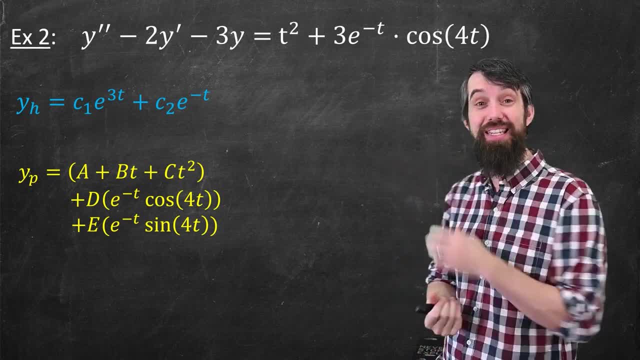 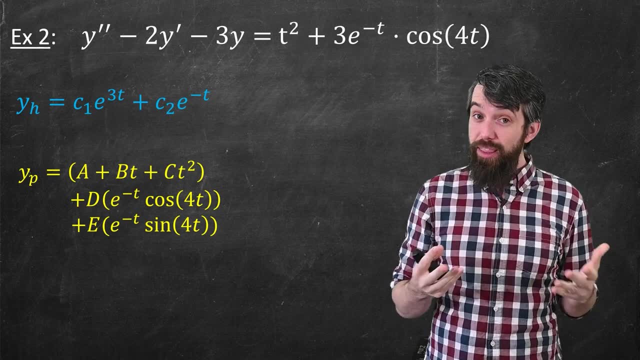 And it could be quite a mess to go and evaluate and I didn't even test to see how messy it would be in this particular case. But it would just be algebra even if it is messy. So you could in theory go and solve for the a, the b, the c. 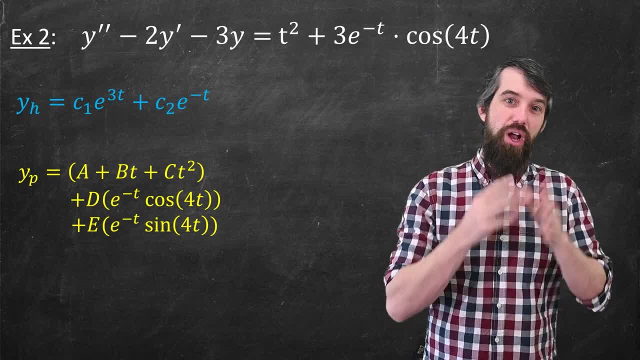 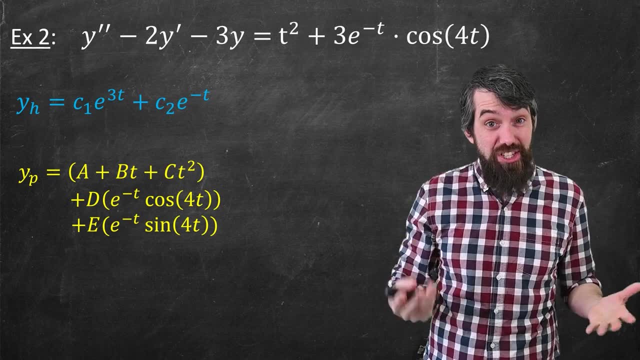 the d and the e, and then you would know your particular final answer: homogeneous plus particular, All right. So I hope you enjoyed this video. If you did, please give it a like for the YouTube algorithm. If you have any questions, leave them down in the comments. 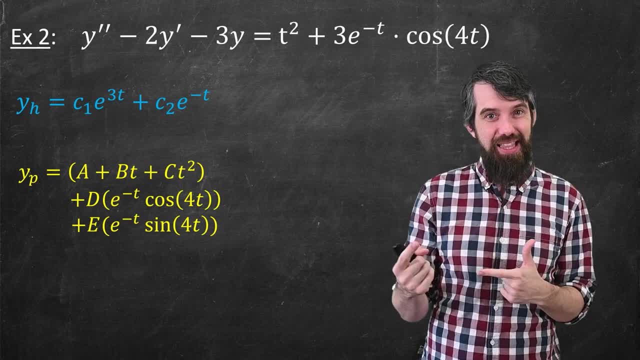 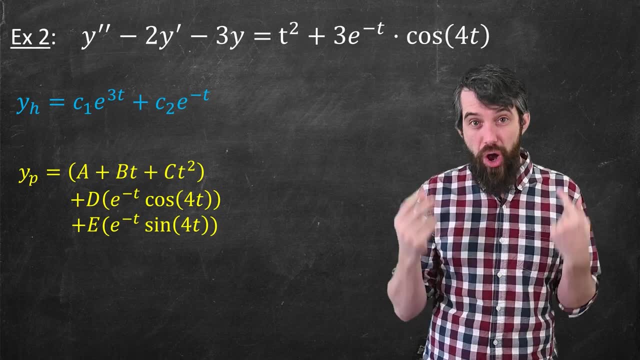 Then for the exponential times, the cosine. we've seen that if there's a cosine term you have to have a cosine plus a sine term. So I'll do that: A constant d times the exponential cosine of four t and then a constant e times the exponential times sine of four t. You have to have both the cosine. 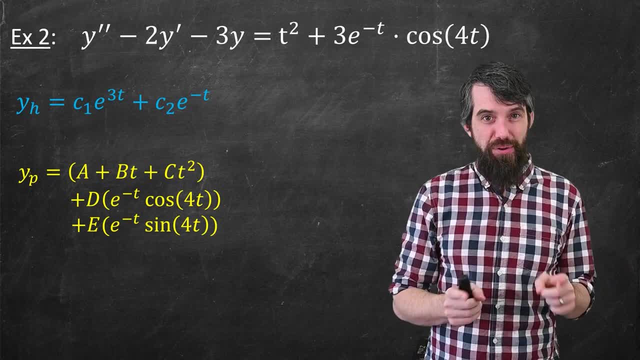 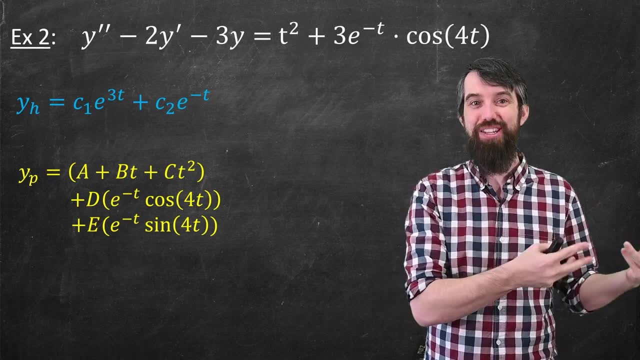 and the sine term added together with different coefficients. Final note is that if it was just e to the minus t without the cosine, you have to have a cosine plus a sine term added together with cosine. You would have had to multiply by the extra value of t, so you didn't match. 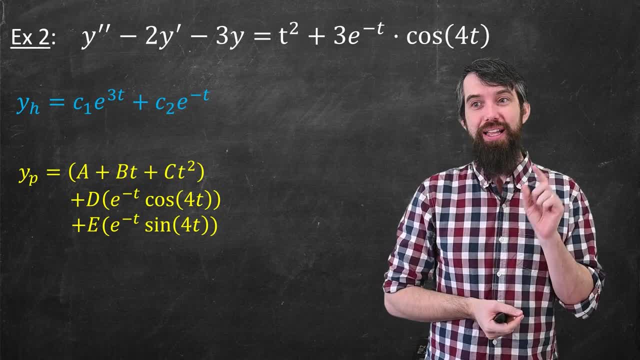 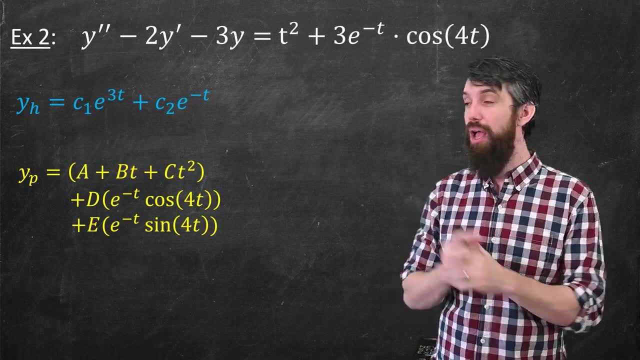 the homogeneous, as I did in the previous example, But here e to the minus t times cosine. that is not a solution to the homogeneous, and so there's no need to multiply by any extra t. So that would be my guess. Now, if you plug it in, there's. 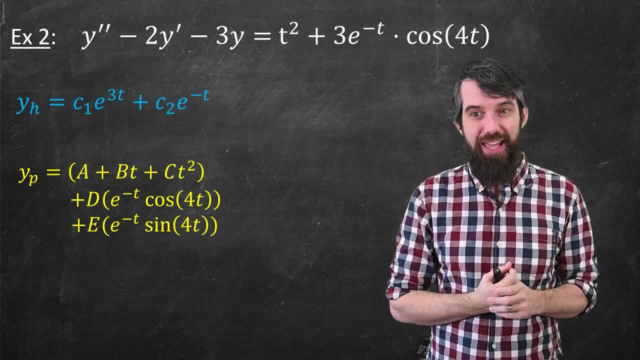 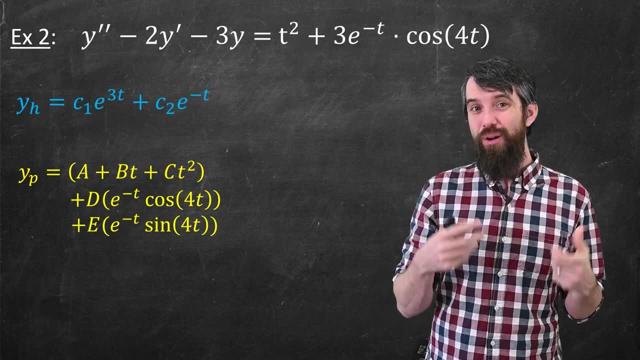 gonna be five different variables- a, b, c, d and e- and it could be quite a mess to go and evaluate them. I didn't even test to see how messy it would be in this particular case, But it would just be algebra even if it is messy. So you 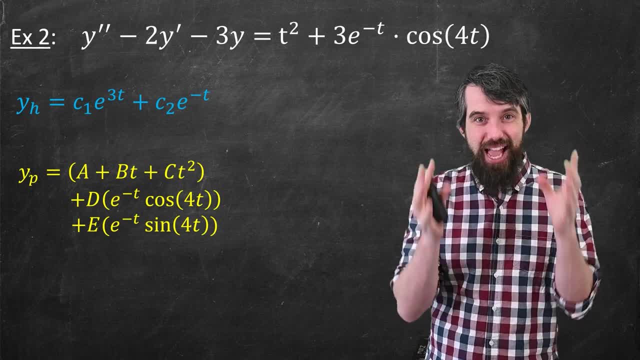 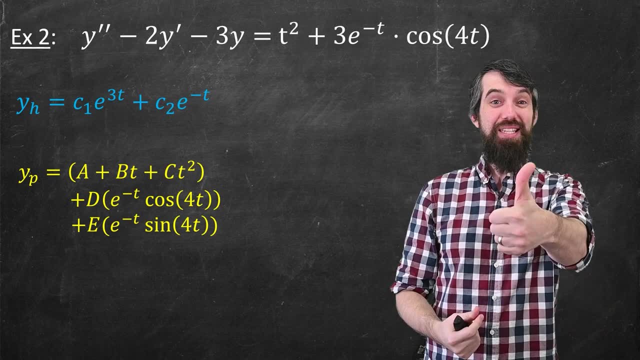 could in theory, go and solve for the a, the b, the c, the d and the e, and then you would know your particular final answer, homogeneous plus particular, Alright. so I hope you enjoyed this video. If you did, please give it a like. 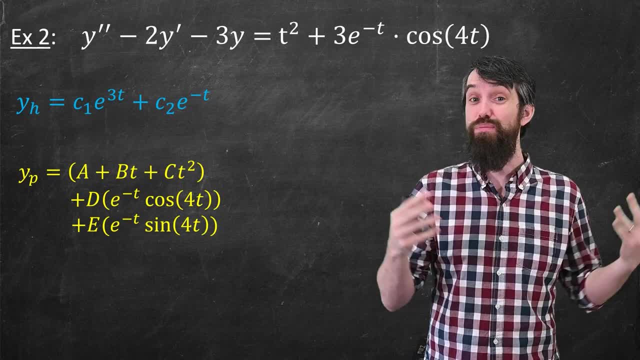 for the YouTube algorithm. If you have any questions, leave them down in the comments below and we'll do some more math in the next video. 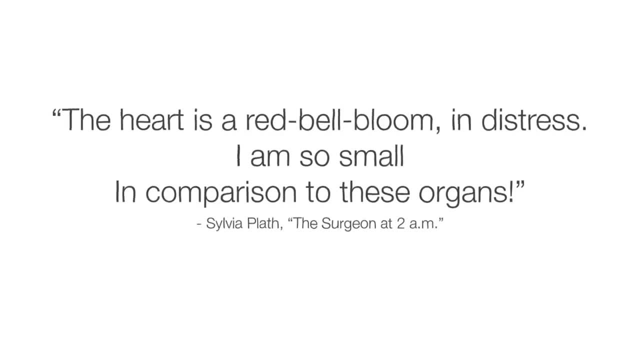 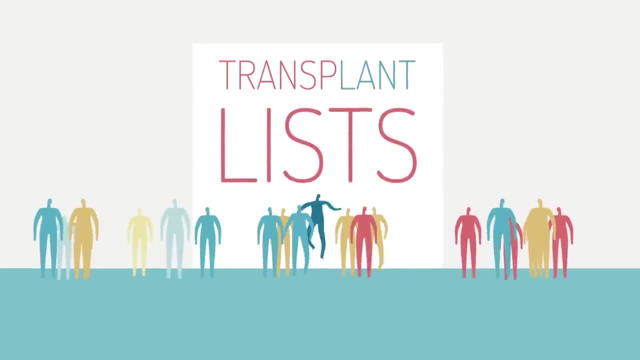 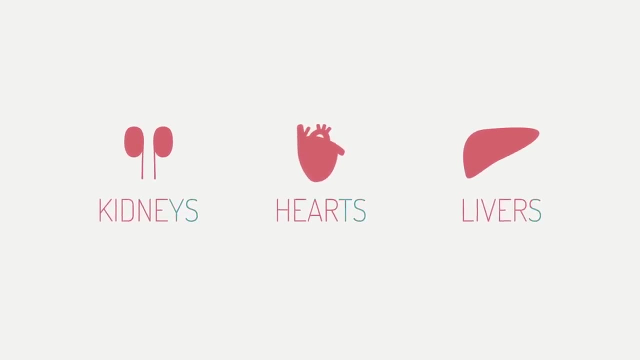 There are currently hundreds of thousands of people on transplant lists, waiting for critical organs like kidneys, hearts and livers that could save their lives. Unfortunately, there aren't nearly enough donor organs available to fill that demand. What if, instead of waiting, we could create brand? 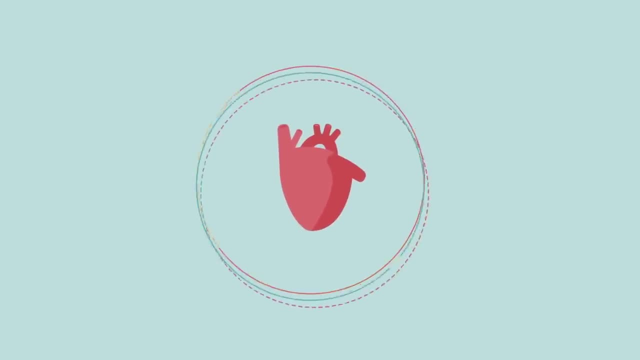 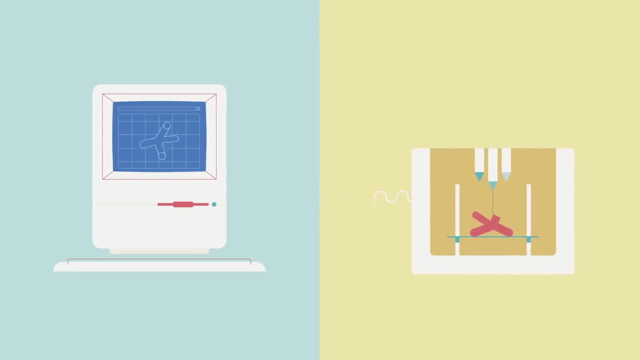 new, customized organs from scratch. That's the idea behind bioprinting, a branch of regenerative medicine currently under development. We're not able to print complex organs just yet, but simpler tissues, including blood vessels and tubes responsible for nutrient and waste.